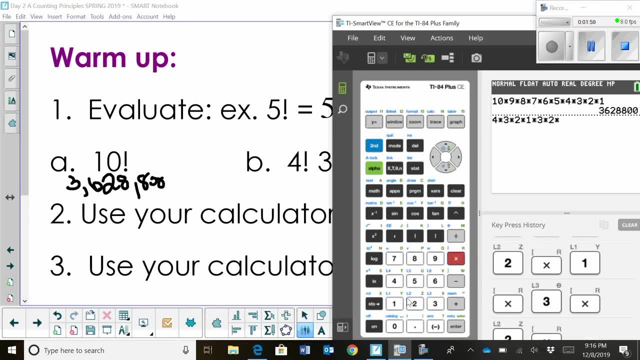 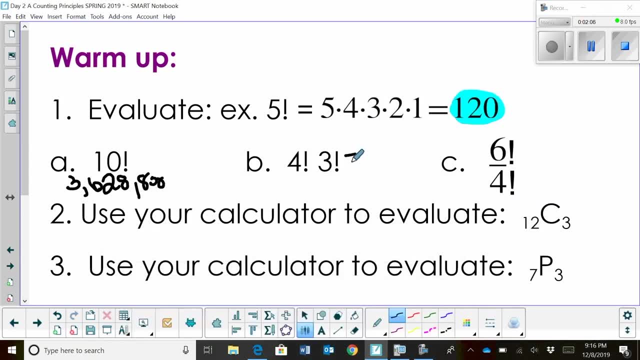 three times two times one, and that gives us 144.. So just hope you're kind of following along how to do this. And then six factorial divided by four factorial. Instead of putting this in the calculator, I'm going to write this one out. Okay, six factorial is six times five. 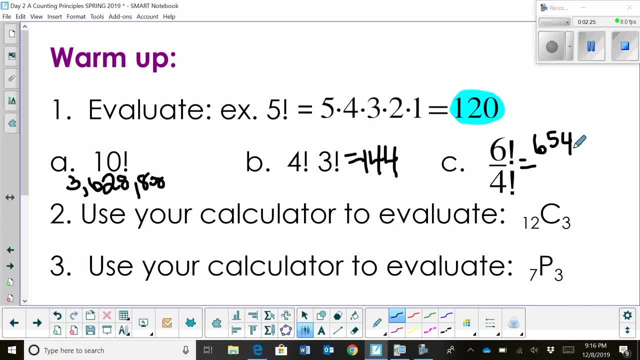 times four, and then four is going to be times three times two times one, So really that's just four factorial. So I have six times five times four factorial all divided by four factorial, which would be four times three times two times one. So guess what Those cancel? 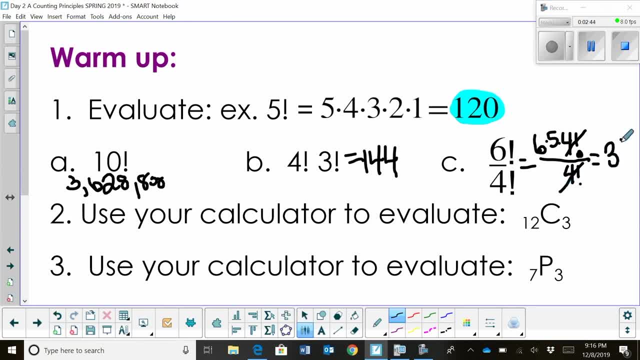 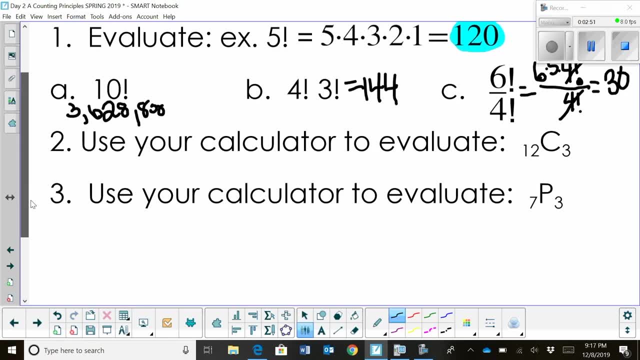 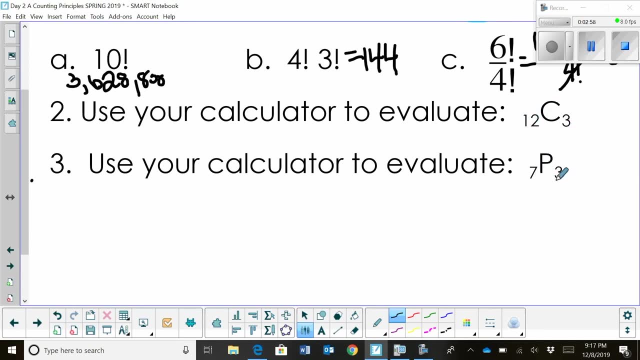 So the answer is just simply 30.. So a real quick way to do it: when you're dividing, you can actually just cancel part of that factorial out. Okay, so now I wanted to show you how to use your calculator to evaluate this. 12C3 and 7P3. 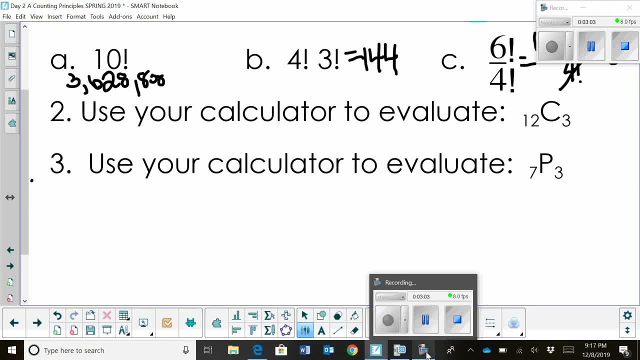 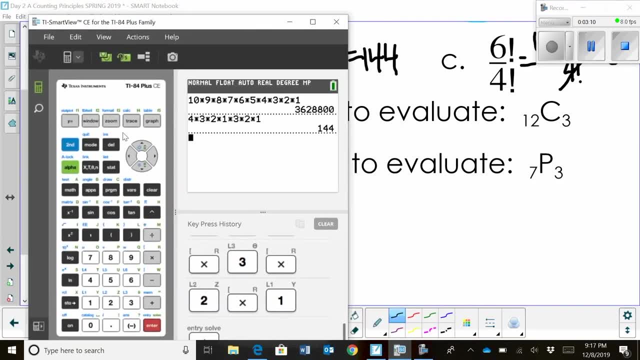 These are combinations and permutations which I'm going to teach you in a few minutes, but I wanted to go ahead and show you how to put those in the calculator so we could just jump straight in. So what you're going to do to evaluate these? you're saying 12 with a combination. 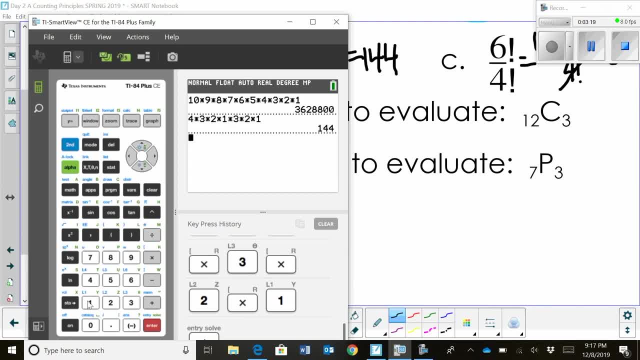 of three. So you're going to type in your calculator 12, then you're going to get a go to the math button and you're going to go over to probability, So math, and then scroll over and you can see the third choice is a combination. So you're going to choose that by hitting enter. 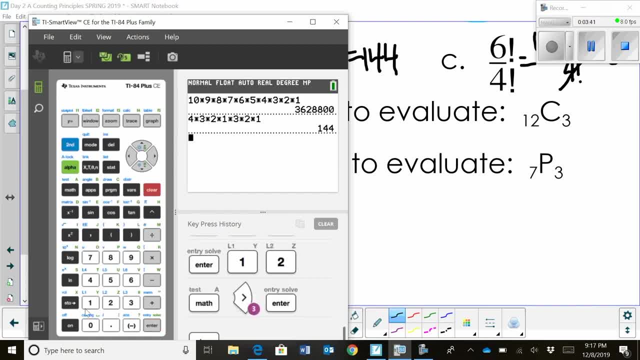 And whoops, something happened there. Let me clear that out and try it again. So 12 math: scroll over to probability. whoops, and I'm going to choose three. I think I went too far, So I'm going to go to probability and I'm going to choose three. 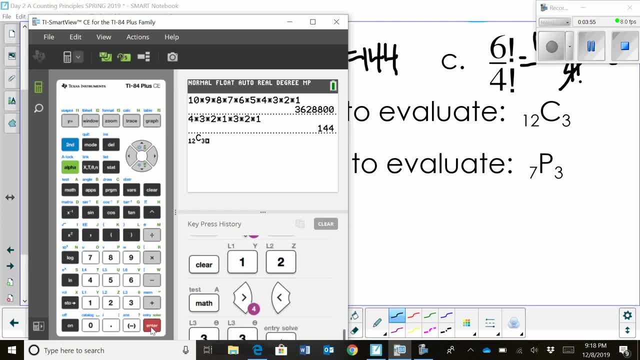 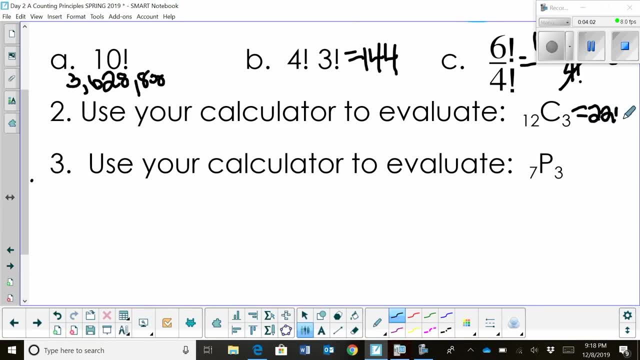 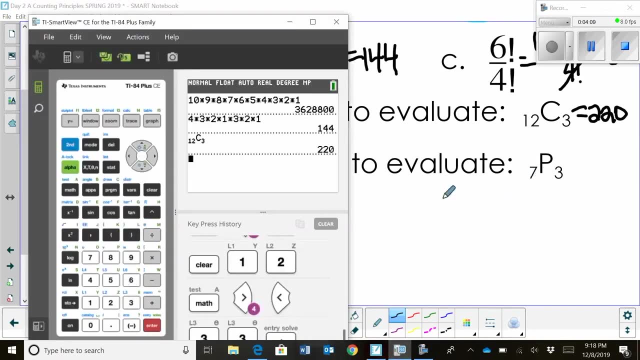 And then choose three. Okay, so that is going to be 220.. Now that involves combinations and permutations, and I'll show you the equation for that when we get to that. And then the second one is a permutation. It is kind of the same concept. You're going to take seven with a permutation. 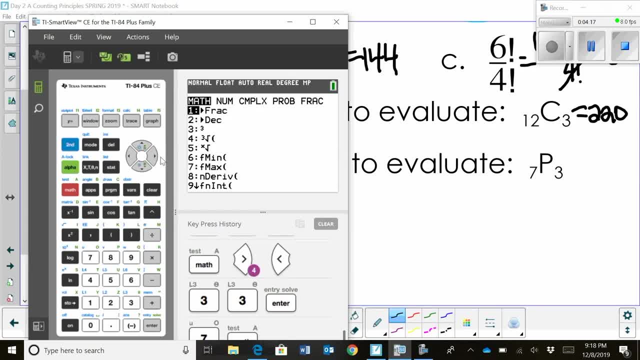 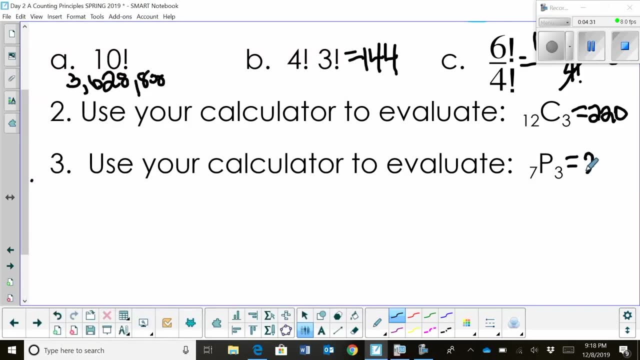 So take your math button after you type in seven, scroll over to probability and this time go to the second choice, a permutation, and we're going to choose three and hit enter, And so that is 221, or two, I'm sorry, 210. And that's how you use your calculator. So those were just some. 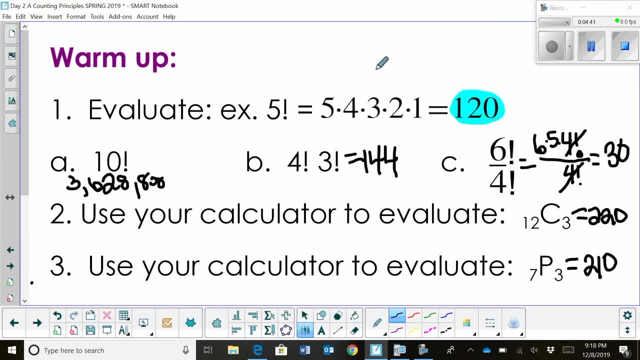 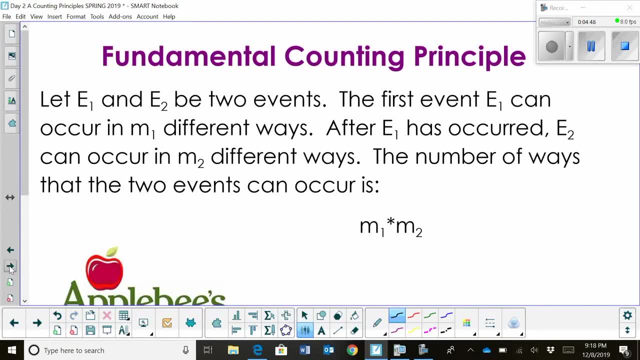 prerequisite skills we needed for this lesson. We needed to know factorials, We needed to know how to type in a combination and a permutation into our calculator. Okay, so let's start with the first concept, which is the fundamental. So let's start with the first concept, which is the 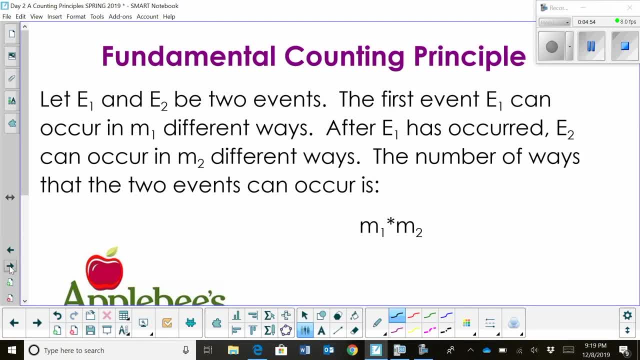 fundamental counting principle. Okay, in this case we're going to have two events. We're going to name those E sub one and E sub two. event one and event two: The first event. it can occur in M different ways, So we're going to use M sub one to refer to the ways that we can count the first. 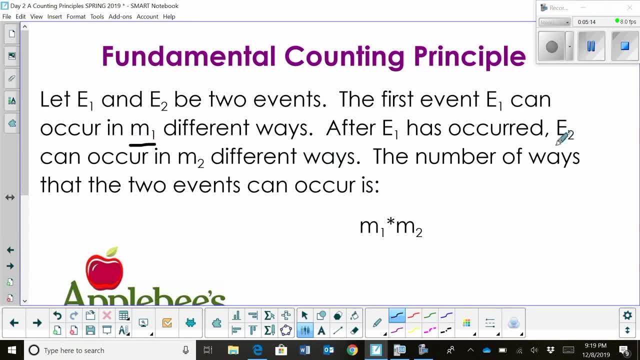 event And then and second event or E sub two occurs in M sub two different ways, And then what we're going to do is we're going to use M sub one to refer to the ways that we can count the second event, And then what we're going to use- M sub two events or M sub two. we're going to use M. sub one to refer to the ways that we can count the first event And then the second event or the third event or the second event or the third event or the third event or the second event, or we're going to use M sub one to refer to the ways that we can count the first event And then along. 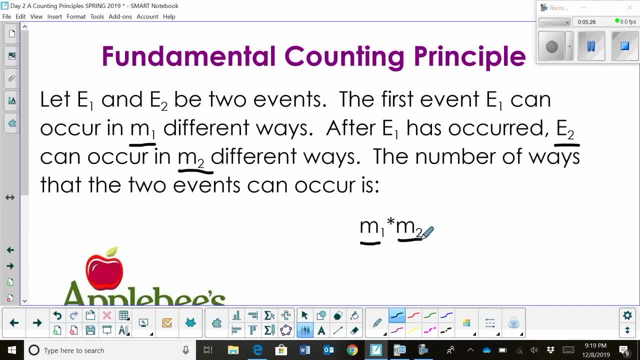 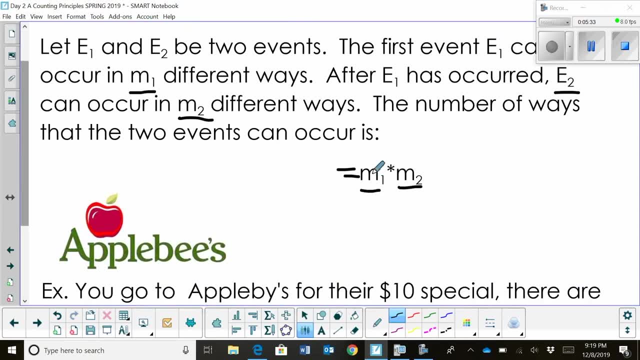 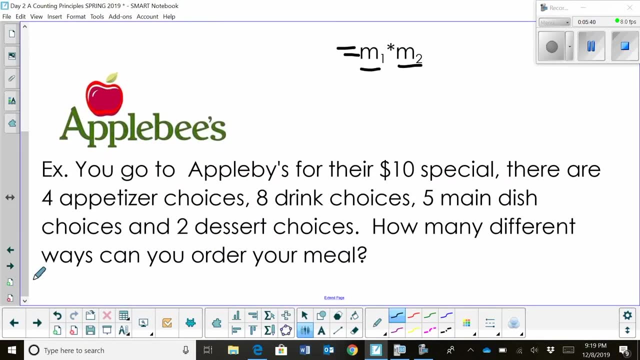 with M sub two, the two events can occur. We would multiply those two different ways together, So the result would be M sub one times M sub two. Okay, so let's look at our scenario so you can see it as an actual problem. It says you go to Applebee's for their $10 special. There are four. 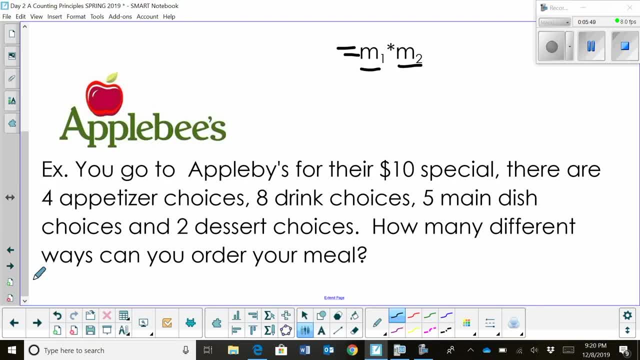 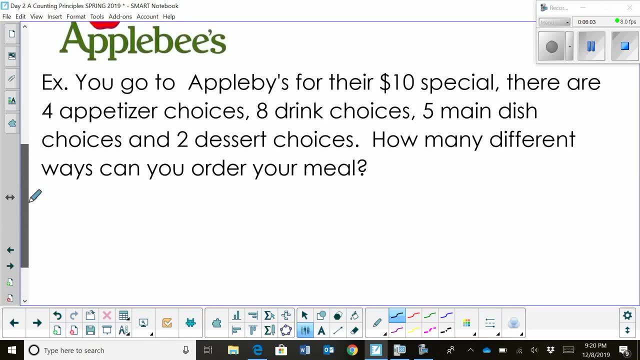 appetizer choices, eight drink choices, five drinks and two drinks. So you go to the珍: five main dish choices and two dessert choices. how many different ways can you order your meal? well, first of all, we need to figure out how many events are occurring. well, in this problem we have 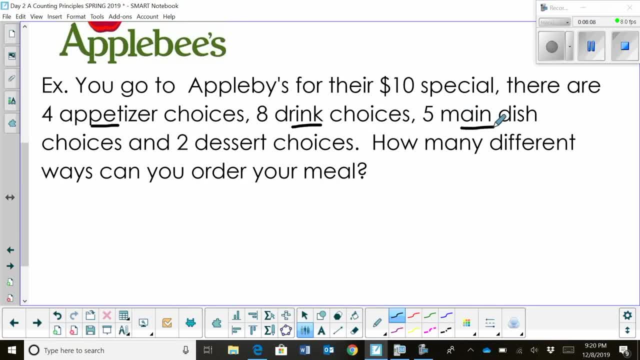 an appetizer, a drink, a main dish and a dessert. so we actually have four events. so what i like to do is just go ahead and draw myself four blanks, one for eat, representing each event. okay, then i'm going to write down my possibilities, how many ways each event can occur. 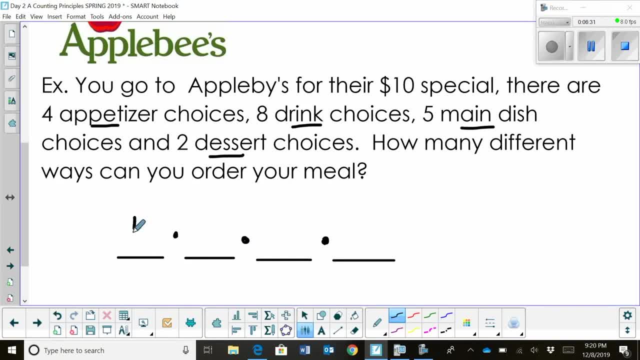 in each of the blanks. so i've got appetizers first, so i've got four appetizers, and then i have eight drink choices. so eight drink choices and then five main dishes, and then i have two desserts. now for the counting principle. all i do is multiply all these together. so let's grab my handy. 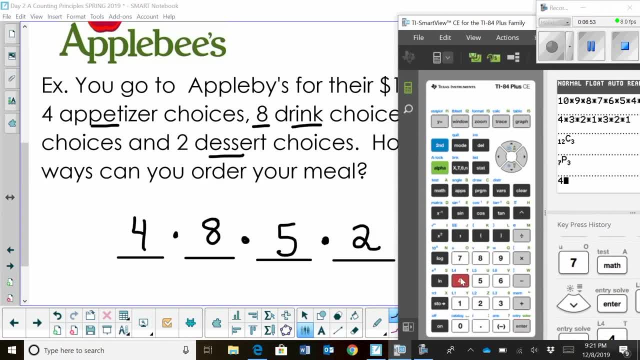 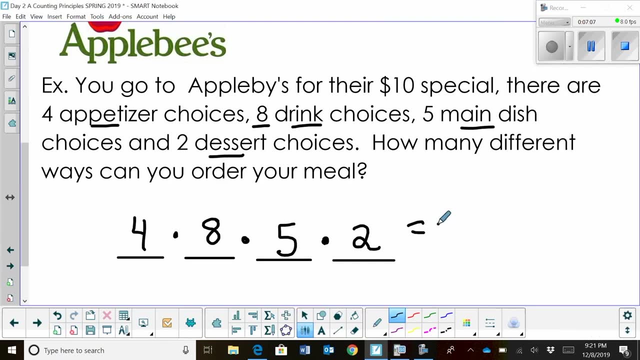 calculator and i'm going to multiply together four times eight times five times two and i get- let me pull this back out- 320 different ways. i can go to applebee applebee's and get a meal, 320, 20 different ways. so i could go almost every day the whole year and get an order from the. 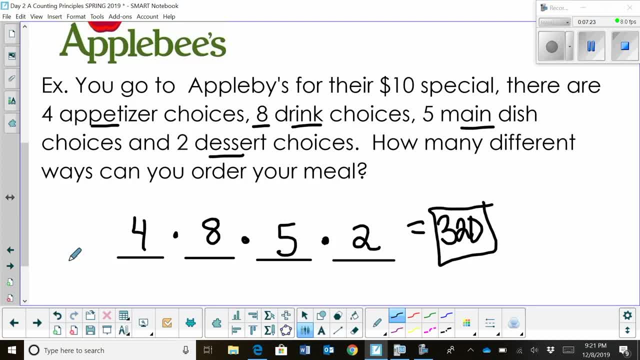 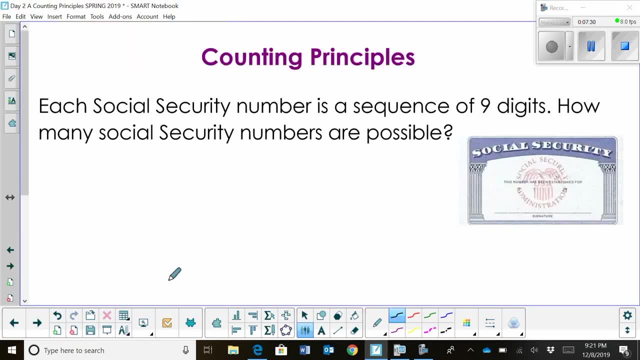 menu and get a different common or different, um different meal every each of those times. so it's kind of interesting to see how many different ways you can do it. so let's look at a couple other counting principles. okay, we've got a social security number pro, i think most. 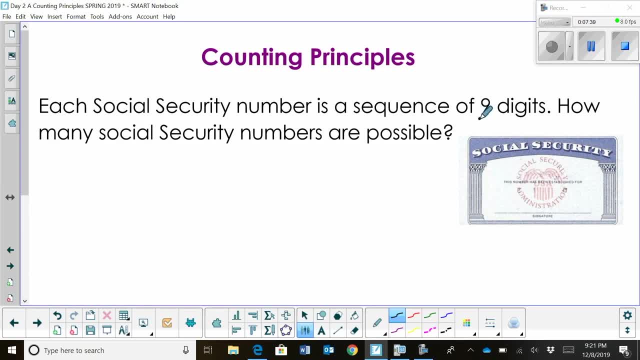 of you have a social security number and there are nine digits in that number. how many social security numbers are possible? well, you have to think. well, how many events do i have going on? okay, so let's say i have nine events, one for each digit. so one, two, three, four, five, six, seven, oops. 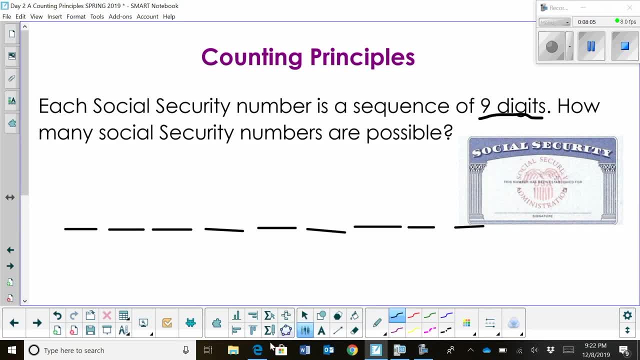 eight, nine, trying to draw straight. didn't draw straight, but that's all right. okay, then you are gonna multiply all these events together. so i'm gonna multiply these and i've got to start thinking: how many different possibilities, how many different ways can i pick the first digit? well, i have the numbers one through nine. 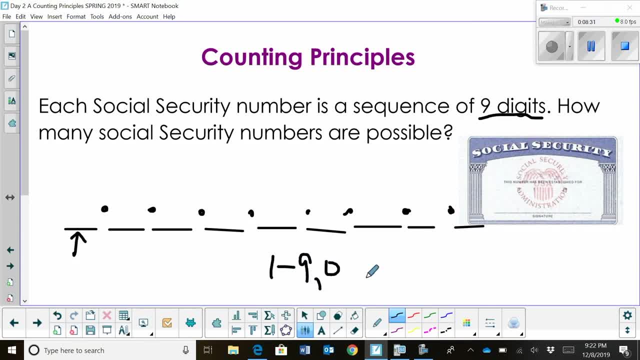 plus, we can't forget about the. a zero, a zero counts also. so you actually have ten different numbers to choose from, including zero. so the first digit could be zero. it doesn't say it can't be. so i have ten choices. well, how many choices do i have for the, my second digit? i have ten more. 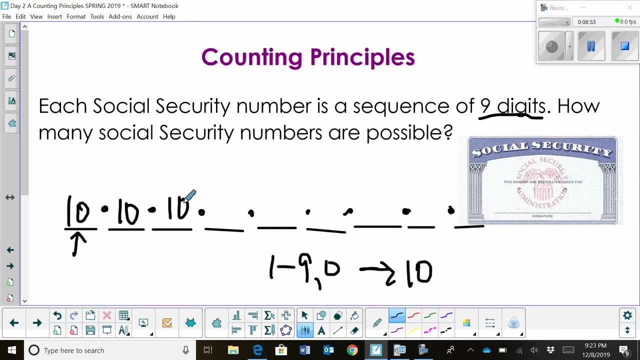 choices, because i can repeat numbers. so i'm gonna have ten choices for all nine positions. so it's just gonna be ten times ten times ten, nine times. okay, we can also write this as ten whoops to the ninth, power, ten to the ninth. so let's grab our calculator and pull that. 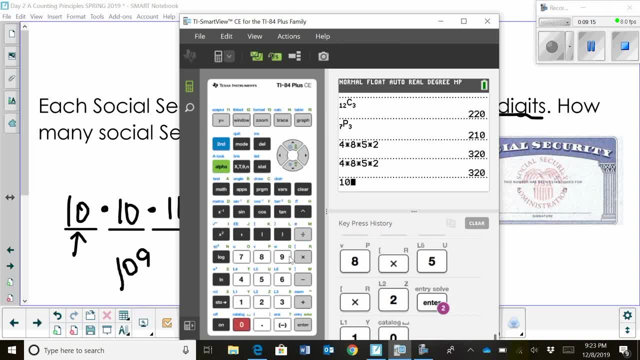 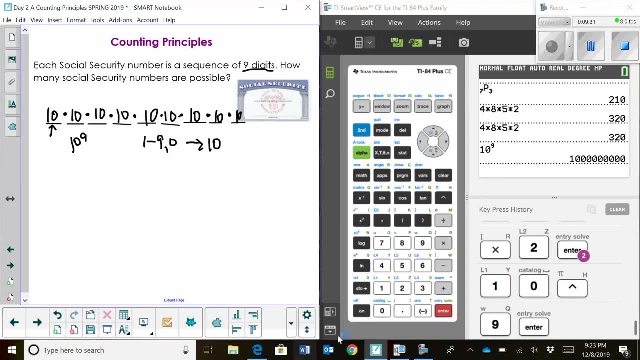 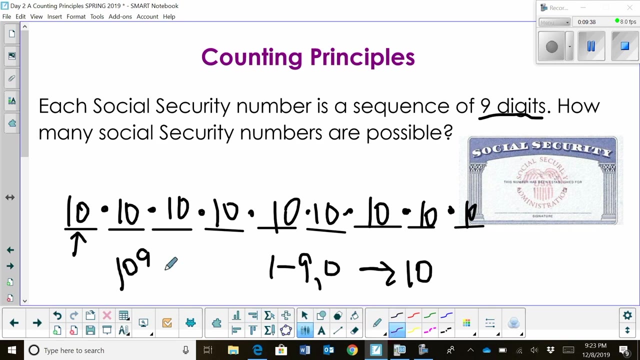 back out and we'll actually figure out how many social security numbers can be created. it's gonna be a lot, wow. so i've got one with one, two, three, four, nine zeros after it. okay, so let's write that net. sorry about that. um, let's grab my pen here- oops, my pen. and i've got one: one, two, three, four. 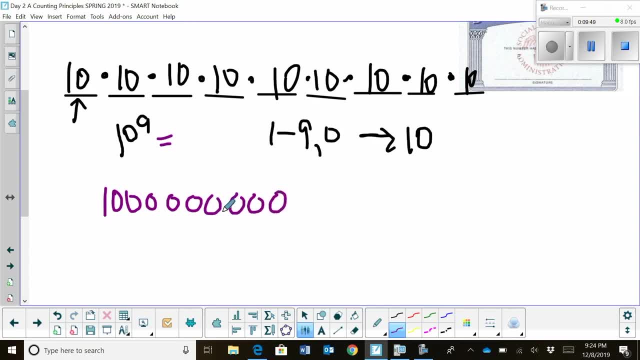 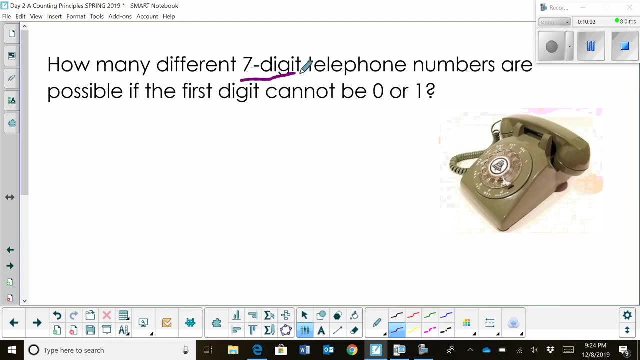 five, six, seven, eight, nine. so what's that? a billion different numbers. we have one billion different ways to get a social security number. so that's a lot. okay, let's try the phone number problem. okay, we have a seven digit phone number. how many are possible if the first digit cannot be a zero or one? we know if it's a zero, that's. 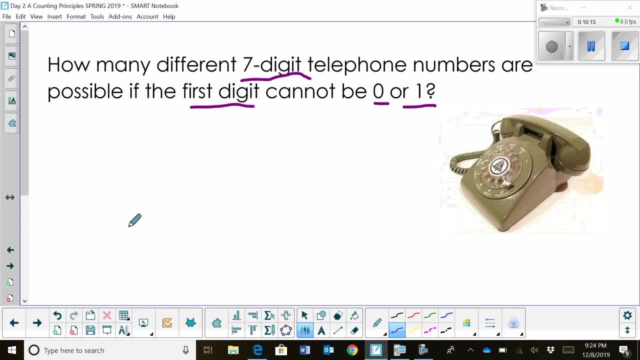 going to call the operator, and if it's a one, it's going to call long distance. so we have to eliminate those choices. so how many events do we have going on? well, we have three in the front, then we usually have a dash here and then four in the back, so we 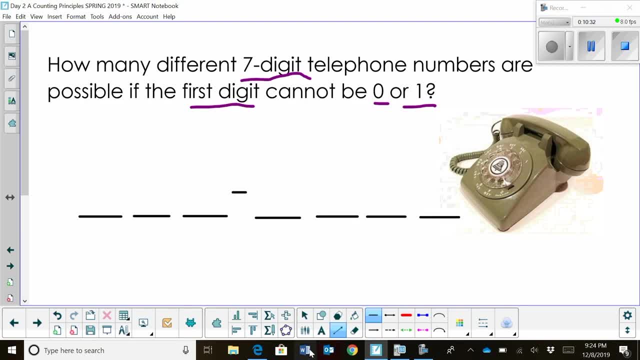 have seven different positions or seven events. how many are how many possible outcomes? or how many ways can i pick the first digit if i can't use a zero or a one? well, that means i normally have ten, but i'm taking two away, so i only have eight choices, but then for the second position, i have ten. 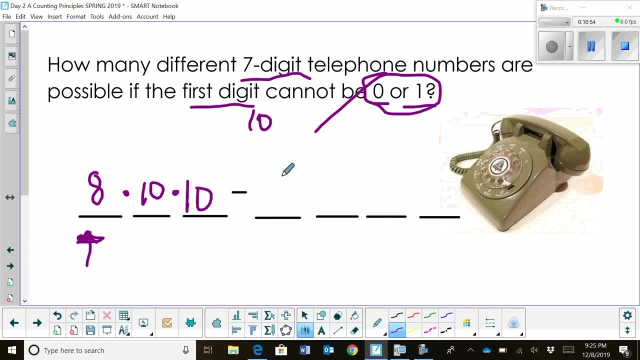 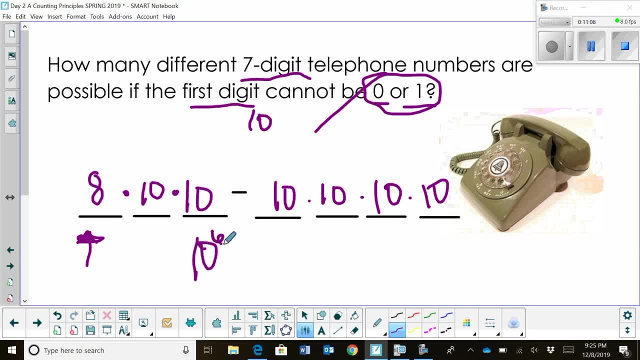 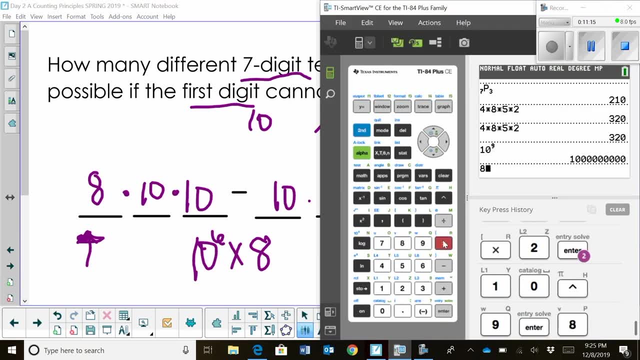 6 power all times 8. so what's 10 to the 6 times 8? let's take 8 times 10 to the 6 power and boom. i have what's that? one, two, three, eight million different ways. yep, eight million, that makes sense, i would. 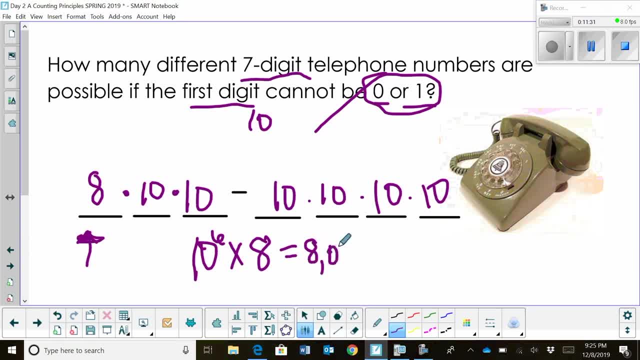 have eight million different phone numbers. now, as you know, there are probably more than eight million phone numbers in the world, so we have to add area codes. that are three digits, and that adds a whole bunch more possibilities. so you could figure that out too, if you wanted to. 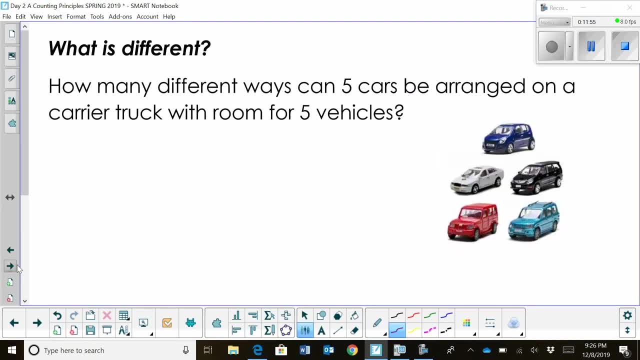 okay, let's see how this problem's slightly different, but we can still use the counting principle. okay, how many different ways can five cars be arranged on a car carrier truck with room for five vehicles? so let's just think about what we have. we have one of these trucks. 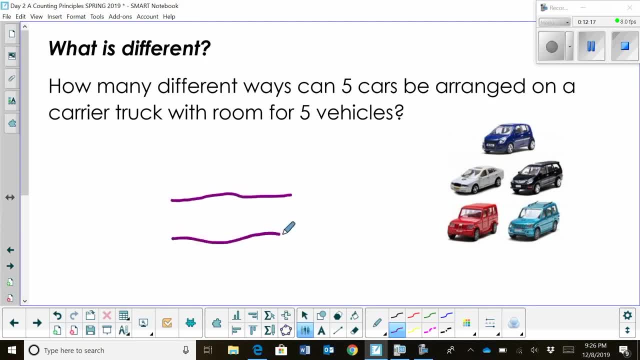 that has a top floor and a bottom floor and then it's got an engine up here. I like to draw a little picture of it, okay, and here's the front light, and here's where the driver is okay and he needs to load. 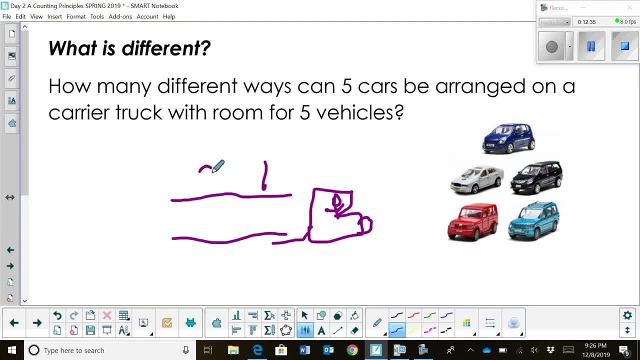 cars up here. Well, we have a spot for one, two, three, four, five cars, something like that. There may be three on top and two on the bottom, but anyway, we have a spot for five cars. How many? 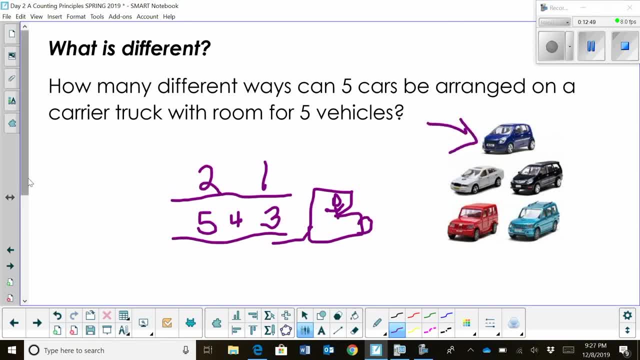 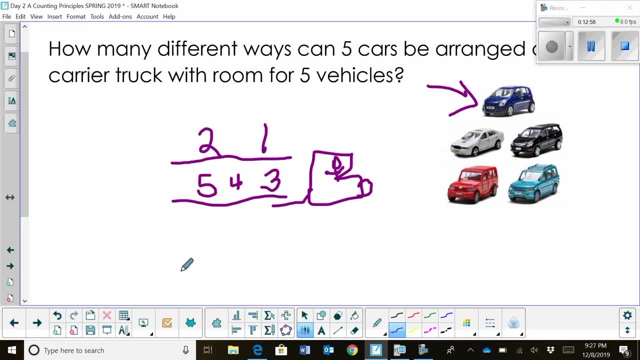 different ways? could we arrange these five cars? Well, what's different about this is, once we place a car, we can't use it again because we've already placed it. so we have to think about our five events. We have five events going on because we have five positions for five cars, so let's draw. 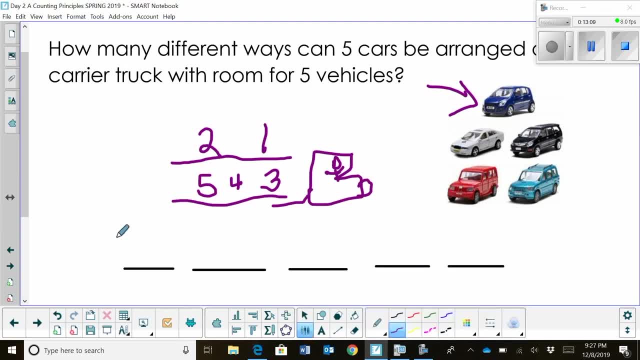 five lines to represent each event. okay, Now for spot one. how many different ways could we arrange these five cars? Well, what's different about this is, once we put a car- let's just say we put the little blue car up there- we now have four choices, and then, once we put a car up, let's say, we put the red one next, we would then have three choices, and then two, and then one. so really, what we've done is we've created a fact. 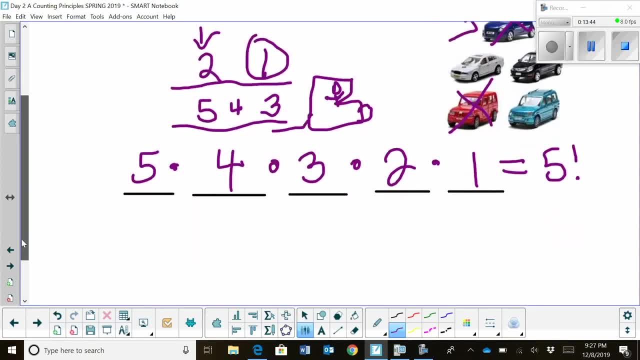 box factorial. Well, what's five factorial? Well, I'm not going to grab my calculator, because this one's pretty easy- That's going to be 20.. And 20 times 3 is 60. And 60 times 2 is 120.. So I have 120. 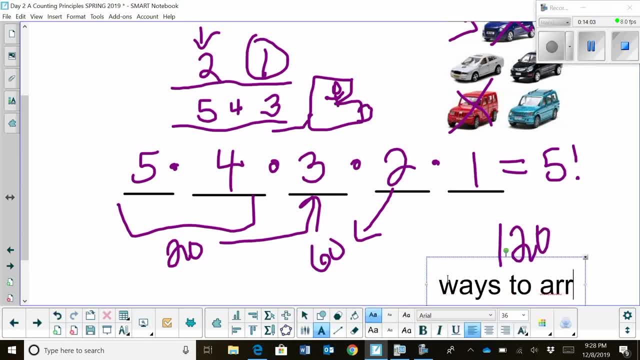 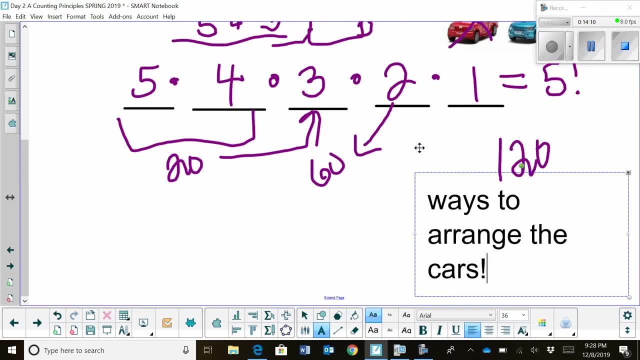 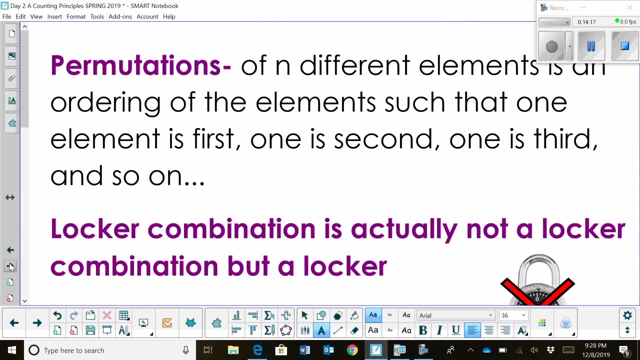 different ways to arrange the cars. That's how many different ways I've got. So there you go. We got 120 different ways to put them on the truck. Okay, So that's kind of the end of the counting principle. Now let's look at permutations. A permutation is a similar situation. It's the. 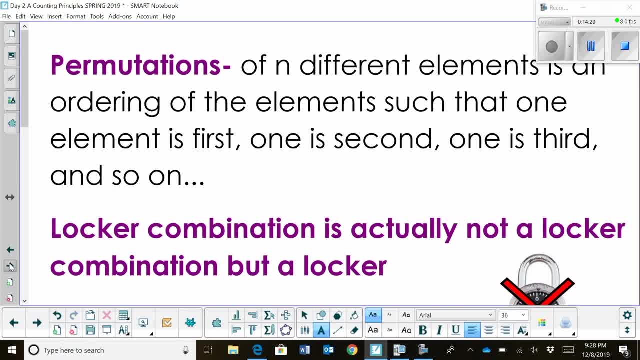 number of different ways of ordering elements, such that one element is first and one is second and one is third, and so on. So it's similar to placing the cars up there as we did in the counting principle, But each one has a spell specific position. So really you could look at the car placement almost as a permutation. Now in the 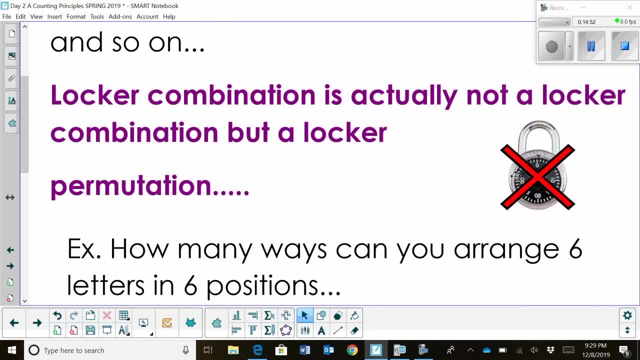 past. I like to relate this permutation to a locker combination. Okay, a locker combination is actually not a locker combination, It's a locker permutation. And why? Because the order that you turn, the dial on the locker, on the lock, the order matters. So if you have, let's just say, your locker combination, 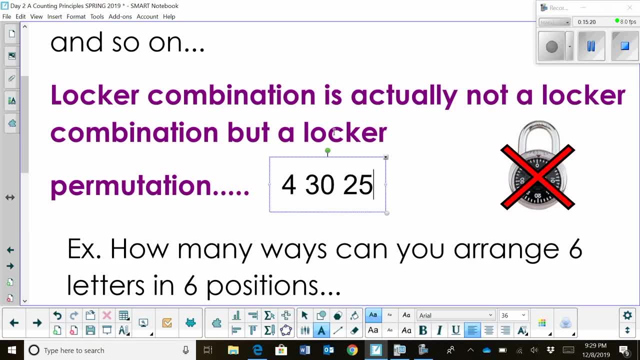 is 4,, 30, and 25.. You have to put it in that order or your locker is not going to open. You can't make it 25,, 30, and 4, or 34 and then 25.. It has to be in that order. So a permutation. 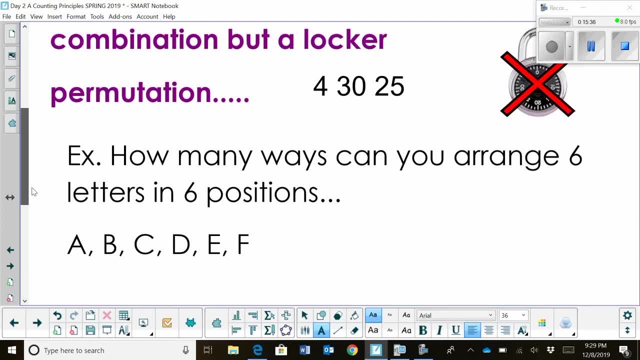 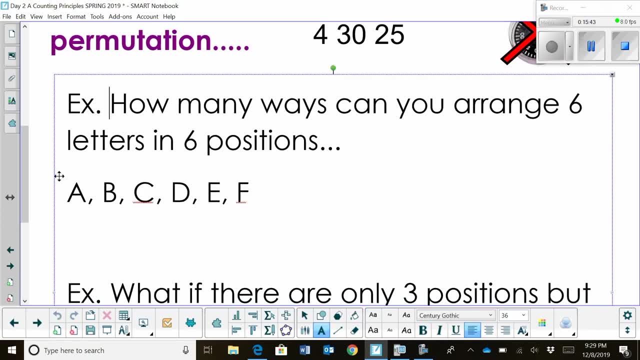 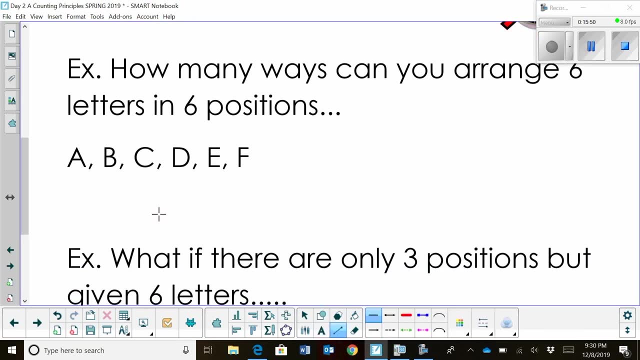 is actually the counting principle, but order matters, Okay. so let's look at this one. How many ways can you arrange six letters in six positions? So in this case I've got six letters: A, A, B, C, D, E, F, But I've got. that means I have six events going. 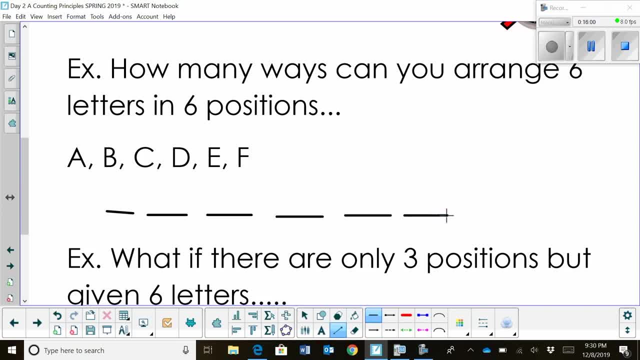 on. so I'm giving myself six spots. Okay, I'm gonna multiply each one of these spots together. but I gotta think: well, how many different ways can I choose my first letter? Well, six, I have six choices, But once one's placed, I have five, then I have four, then I have three, then I have two, then 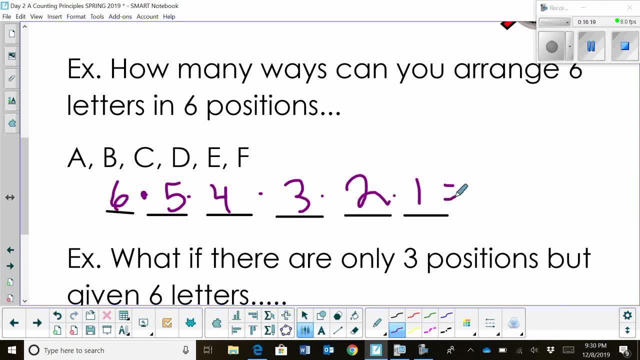 I have one. So really guess what that car problem was. a permutation, But it's a type. it's a special type of the counting principle. Okay, so let's multiply all this together. This is going to give me 30 and 34.. 30 times 4 is 120. And 120 times 3 is 360. And 360. 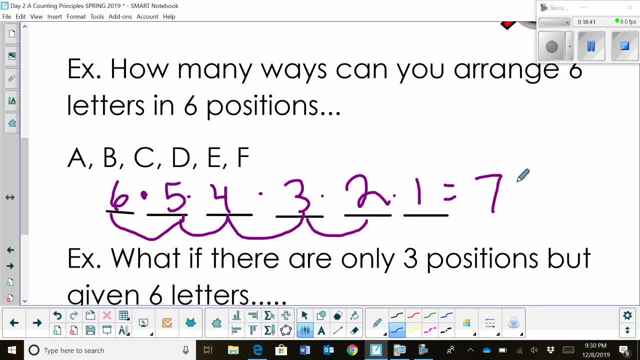 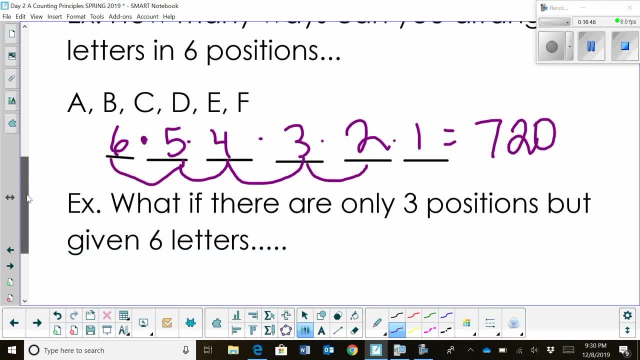 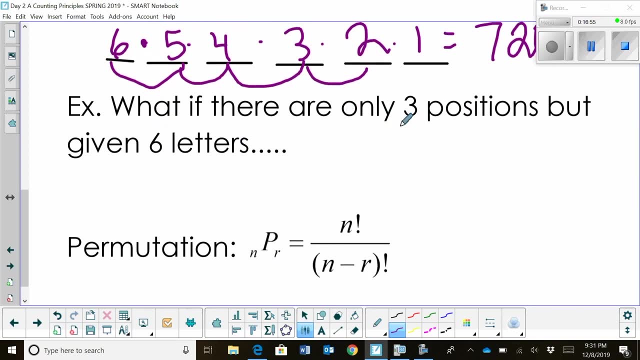 and 360 times 2 is 720 different ways that we could arrange the six letters into different combinations, different patterns. Okay, now let's look at this one. What if there were the same six letters but we only choose three of the positions? What if, instead of having six events, we only have? 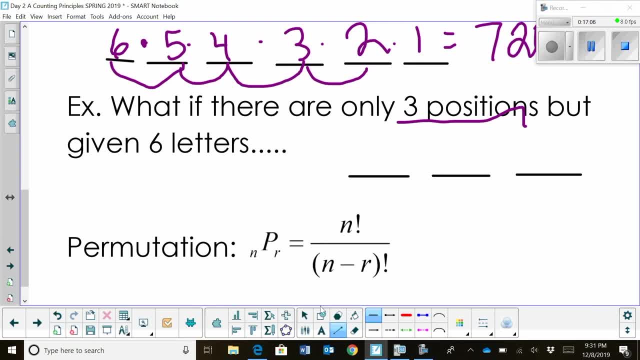 three events. Well, that's going to change things. Okay, so we have: for the first choice, we still have six. For the second choice, we have five. For the third choice position, we have four choices. So really, we only end up with 30 times 4, which is 120 different. 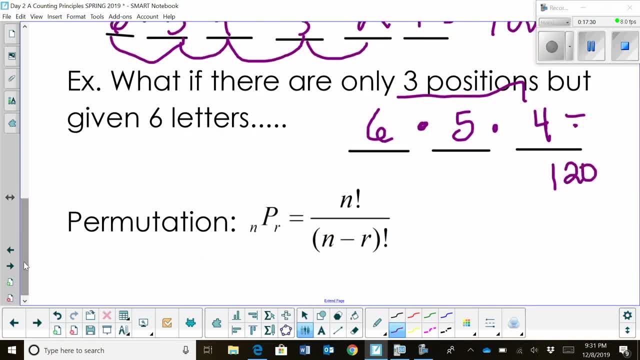 ways to choose those letters. We can use the permutation equation to figure that out. Where n is the total number of possible choices. in this case it would be six. R represents how many we're choosing, How many positions we have- In this case this one's three- And then we plug this into a factorial equation. 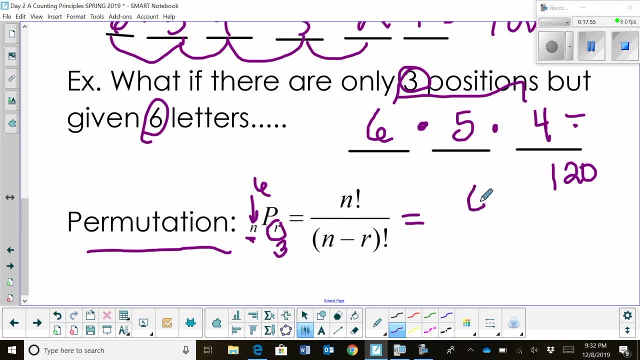 Where we have n factorial, where n is six. So let's write six factorial over six minus three, which is n minus r, all factorial, to take the difference between the two and take that factorial. So in this case we have 6 factorial over 3 factorial. Well, earlier, remember how I showed you how to do factorials. 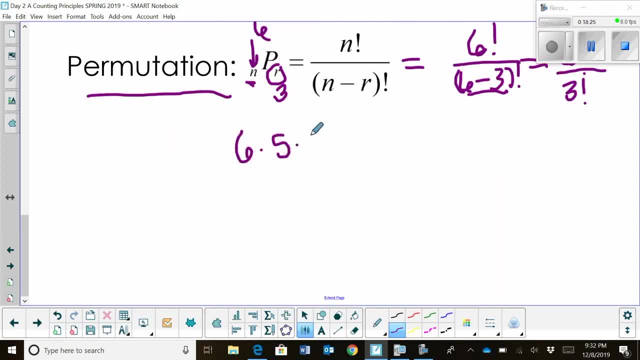 So is that 6 factorial 6 times 5 times 4 times 3 to 1, which is just 3 factorial all over 3 factorial. Well, the 3 factorials cancel out and yes, indeed, we got 6 times 5 times. 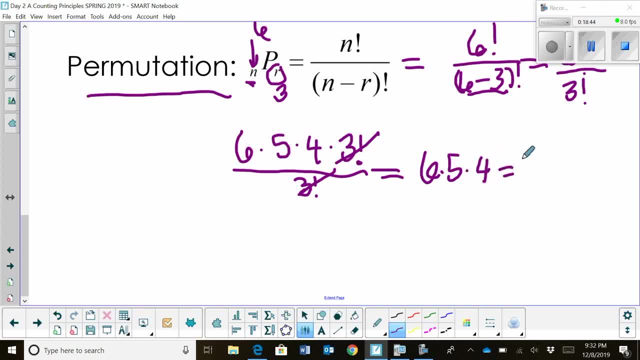 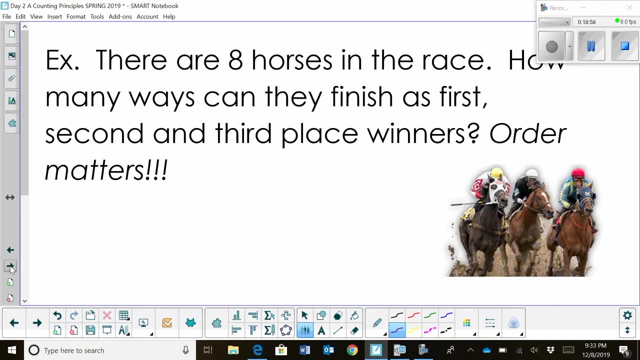 4,, which ends up being that 120.. So you can kind of think of it two different ways. You can use the equation or you can just think about the positions and the possible outcomes. Okay, so here's one. We have to think about positions. There are eight horses in a race. 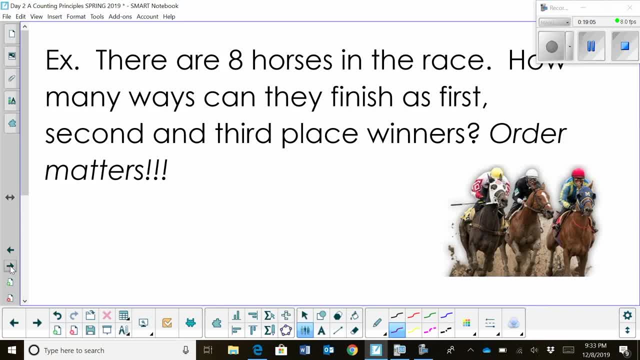 How many horses are in a race? How many horses are in a race? How many horses are in a race? How many ways can they finish as first, second and third place winners? Okay, that order's important. Why is order important? Because you're talking about first, second and third. 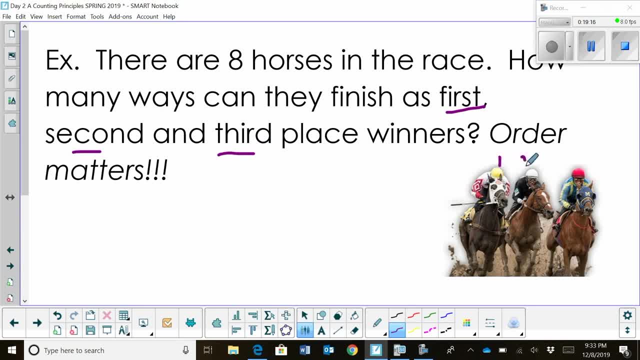 place, So you could have the same three horses finish in a different order, and it makes a new solution or a new answer, a new outcome. So you have to think about that. That's what a permutation is. So let's do it both ways. We'll first do it with the counting principle. 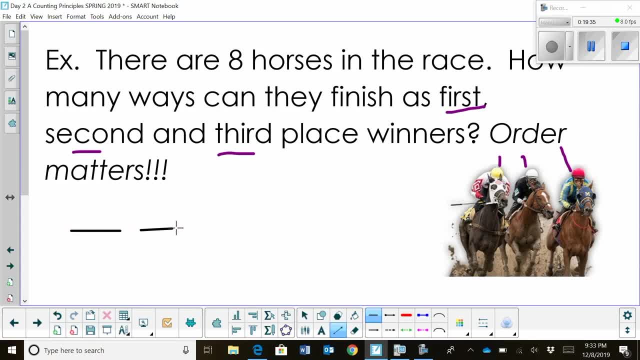 thinking about the events. So we have three events occurring because we have three outcomes: We have a first place winner, we have a second place winner and we have a third place winner. So we have to think about how many choices we have. Okay, those are the events. How many ways? 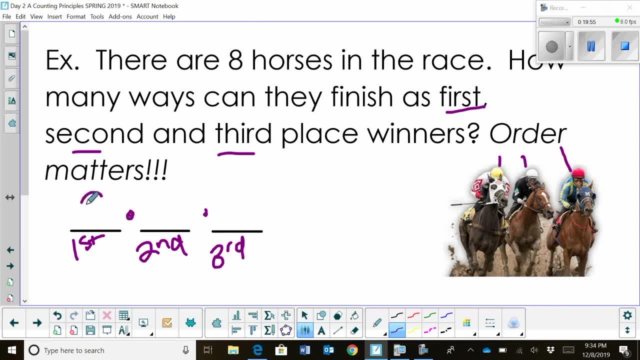 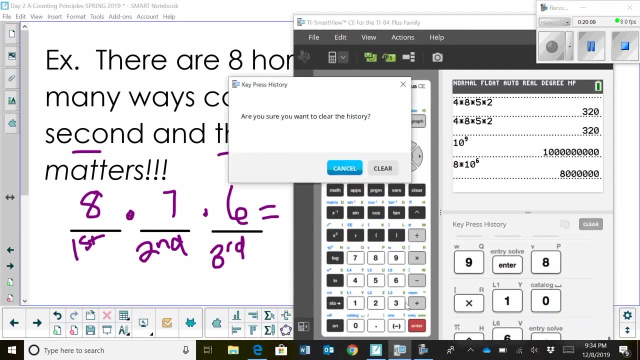 can we have a winner with eight horses? Well, eight choices, How many ways? Once one has won, we have seven choices for the second place And then six choices for the third place. So let's get our calculator out And let's. 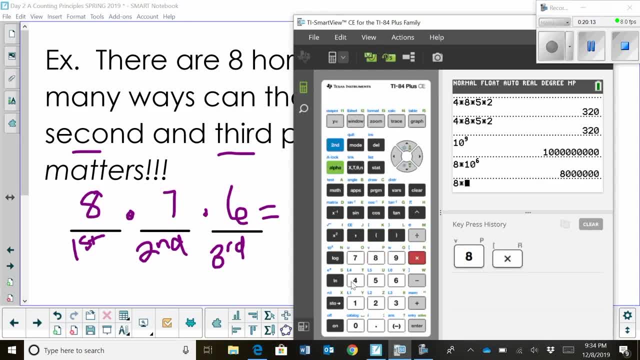 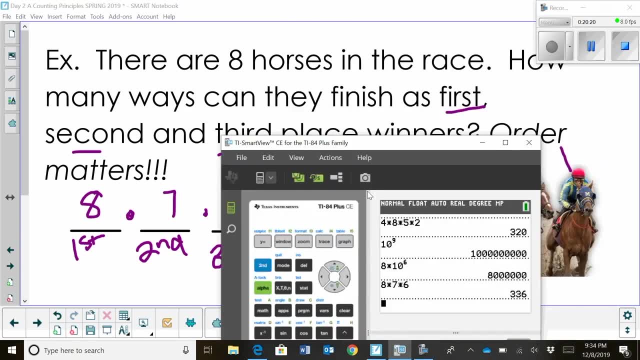 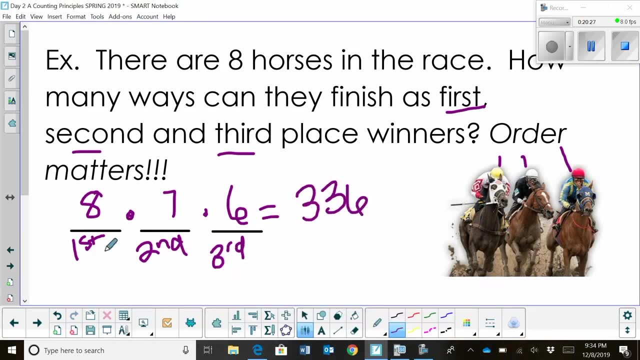 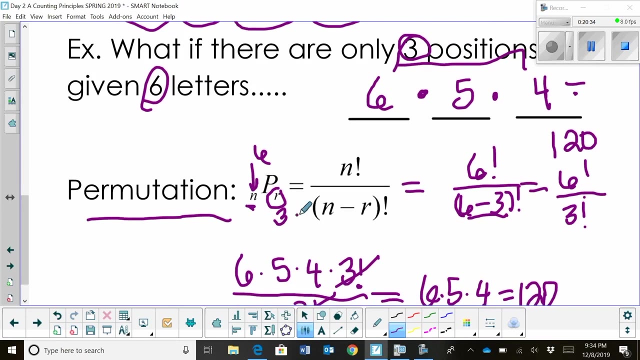 multiply eight times seven times six, And that gives us 336 possible ways those horses can finish first, second and third. Okay, now let's look at it with a formula. Now, here's our formula. I'm going to go back and pull this formula. Okay, I'm going to erase this real fast. so 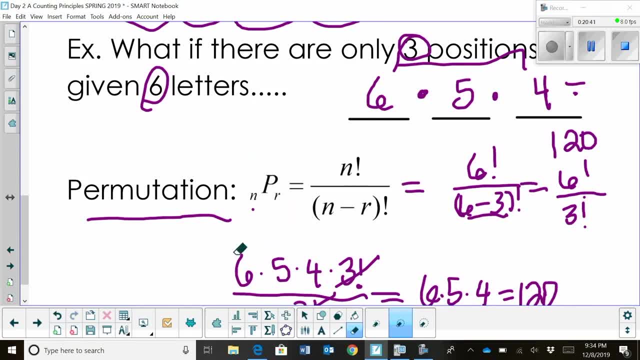 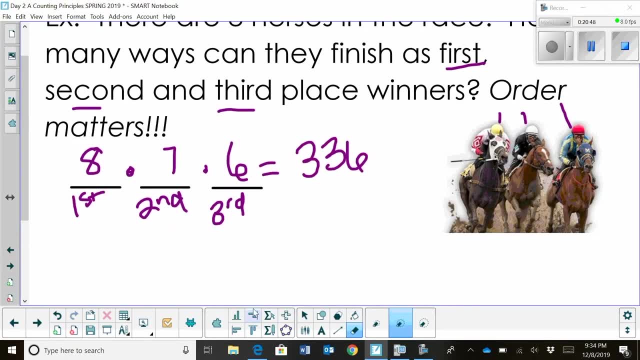 we can look at it a little bit better. Okay, we're going to have n factorial over n, minus r factorial, So I just wanted to show you that. So n, in this case, is how many total do we have? Well, we have eight And we're going to take a permutation because order 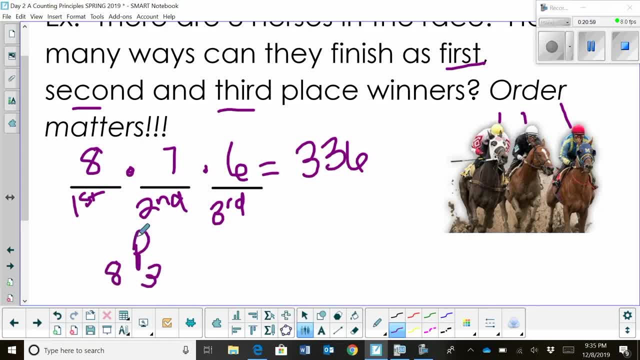 matters And we want three positions. So it's eight permutation three. So we're going to have n factorial over n minus r factorial. So we're going to have three And that means we're going to have an eight factorial which is n factorial. 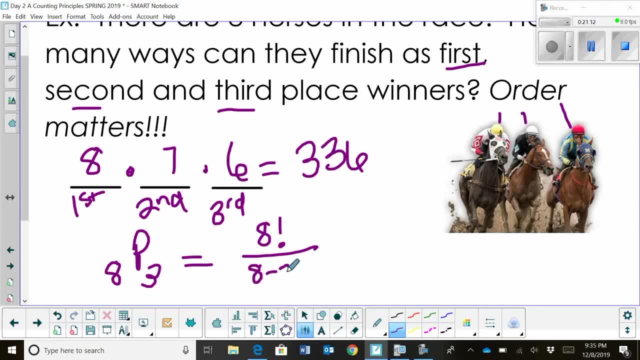 over n minus r, So eight minus three factorial And that gives us eight factorial. I'm just going to go ahead and subtract the bottom so you can see it, And that's five factorial. So really we're just taking eight times seven times six times five, So that's going to be. 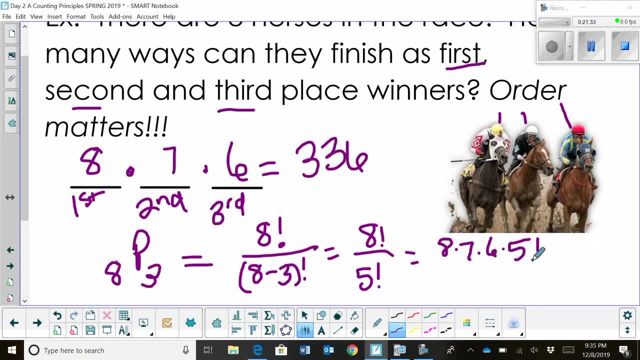 five factorial. Okay, so now, what's the number of horses? Well, we want a number of horses, So we're going to have factorial all over 5 factorial, which cancels. and I have 8 times 7 times 6, which is 336. so when we talk about showing our work, this is actually what 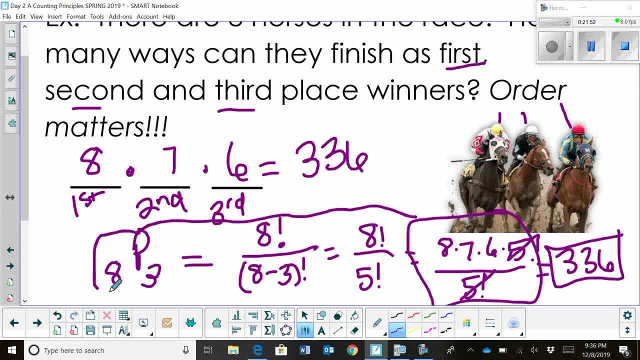 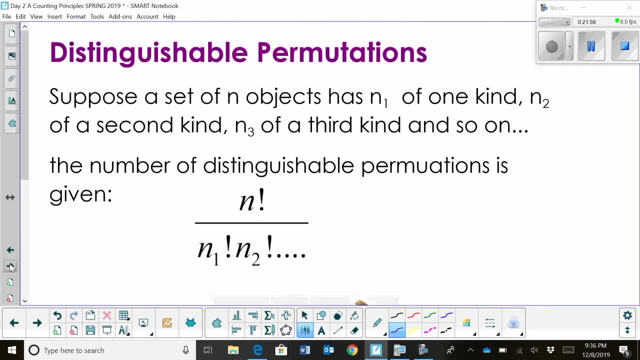 we mean writing the formula showing that we understand what factorials are, and that's how we show our work. okay, now let's talk about a special case of a permutation. suppose you have a set of n objects and some of them repeat there's. so you have n sub 1- one of the objects is one of a kind, and sub 2 there's 2 of. 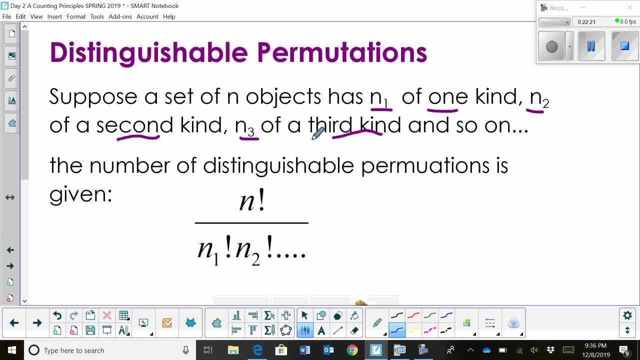 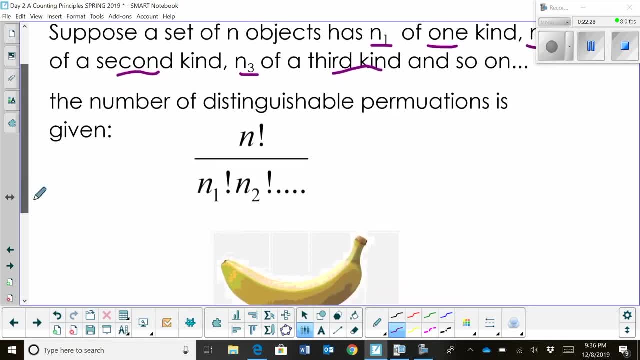 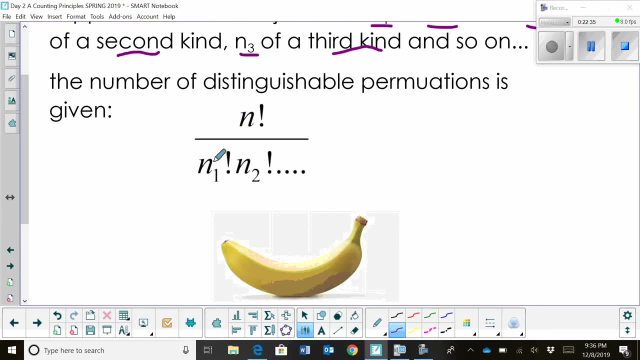 a kind and sub 3, there's three of a kind and so on. so you have repeating objects in a group. okay, to find the number of permutations, we're going to take n factorial, which is the total number of bad operations of all the objects and divided by, in fact, n sub 1 factorial, n sub 2 factorial, or whatever is being. 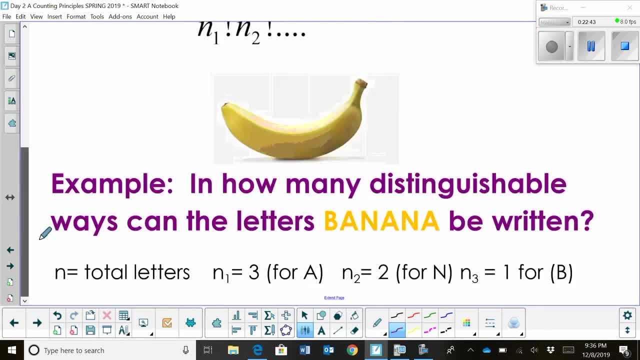 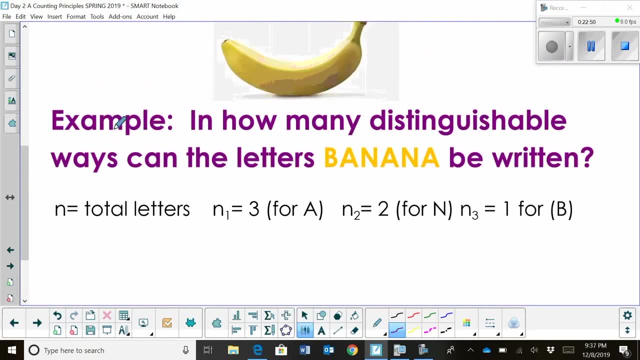 repeated. so let's look at the case of the banana. okay, here's the case of the banana. for our distinguishable permutations, and how many distinguishable ways can the letters banana be written? well, remember, we have in banana one, two, three, four, five, six letters. so for our permutation wouldn't we take 6 factorial. 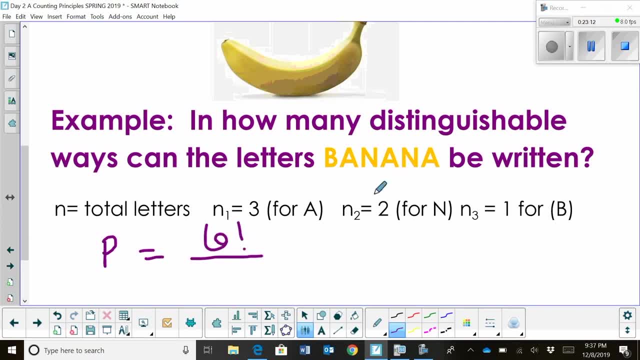 and then we would choose six ways. but because a occurs three times, those positions are not going to be unique, because whether that a is the first day or the second day or the third day, we don't know, those are, those are repeating in our pattern. so I have to divide by three factorial to represent. 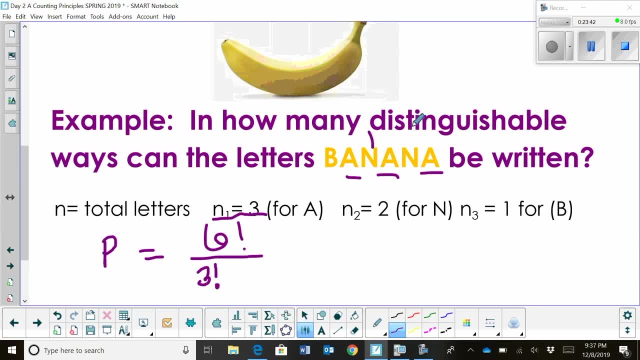 the letter a then, and it occurs twice. so I have to divide by a two factorial because it occurred twice. now the be I don't really have to worry about because it's one letter and it would be one factorial, so that's just one. so So I've got to take 6 factorial divided by 3 factorial and divide times 2 factorial. 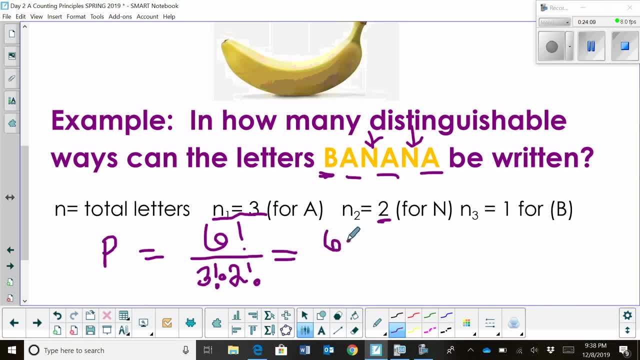 So I'm going to write the entire sequence down. So I've got 5 or 6 times 5 times 4 times 3 times 2 times 1.. And I'm going to divide that by 3 factorial, which is just 3 times 2 times 1.. 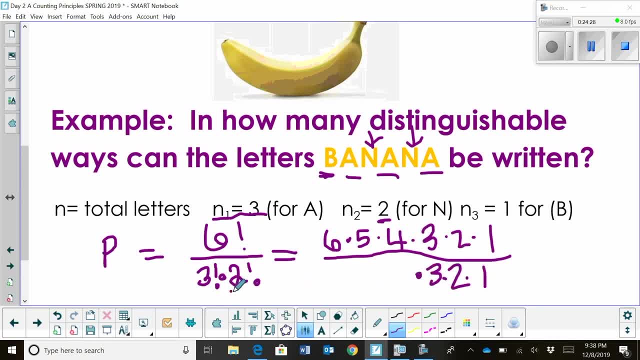 And I'm going to write it under there because I know those can cancel. So I'm going to have another 2 factorial where 2 factorial is 2 times 1.. So I'm going to write that one all out. Now let's cancel out what we can. 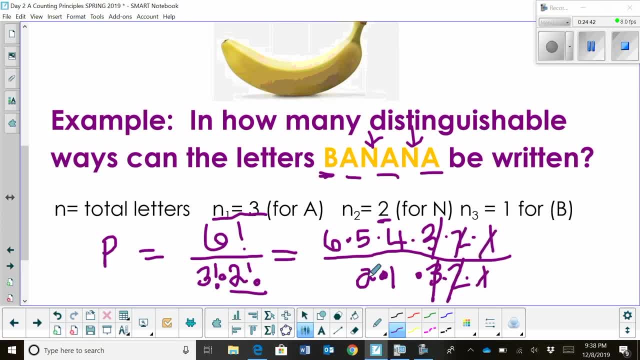 We can cancel the 3s, we can cancel the 2s, we can cancel the 1s, And then 2 does go into 4, so I could reduce this by 2.. And then really, I'm just multiplying together 5 times, 6 times 2.. 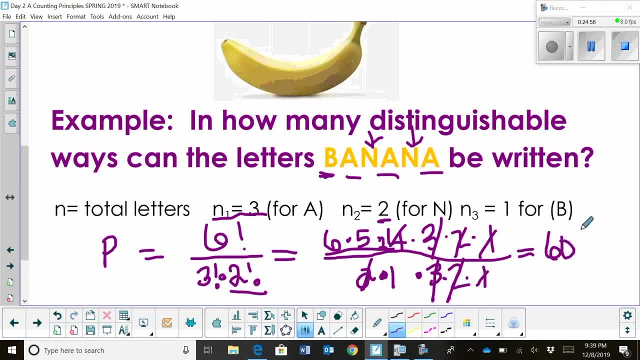 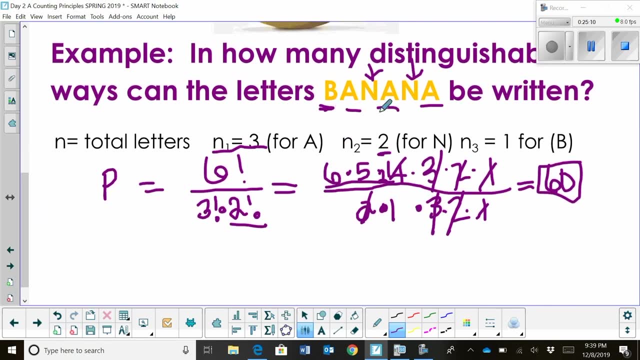 So that's 60 different ways. The letters in the word banana. That can be arranged to make unique patterns of 6 letters And that's how you figure out a distinguishable pattern. So that one's a little bit different because we have to think about repeating choices in. 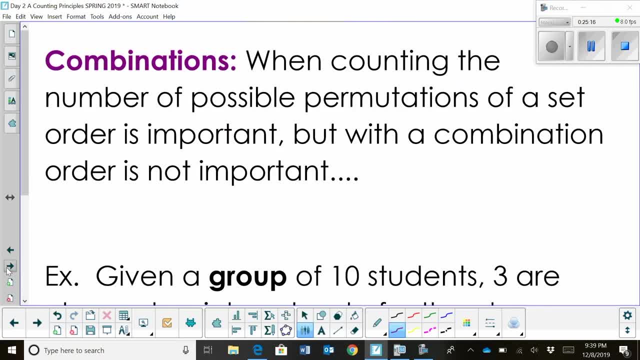 a pattern. OK, so now we're on to the next topic. This one is combinations. So, in probability, you have permutations and you have combinations, as well as the counting principle. So we're looking at our third option, which is combinations. 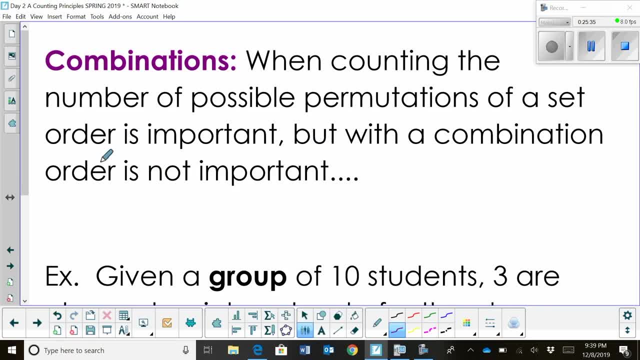 A combination is when counting the number of possible permutations in a set, where order is important, but in a combination the order is not important. So when you're doing a permutation, order is important When you're doing a combination. let me highlight this. 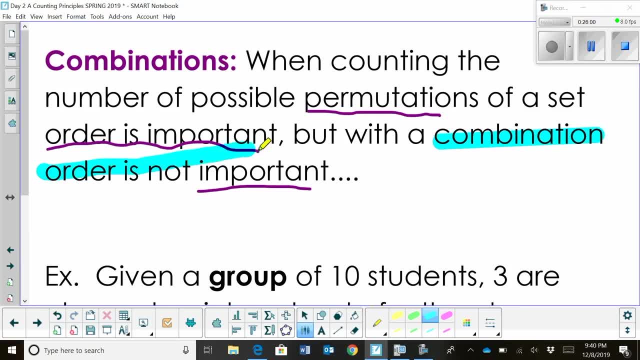 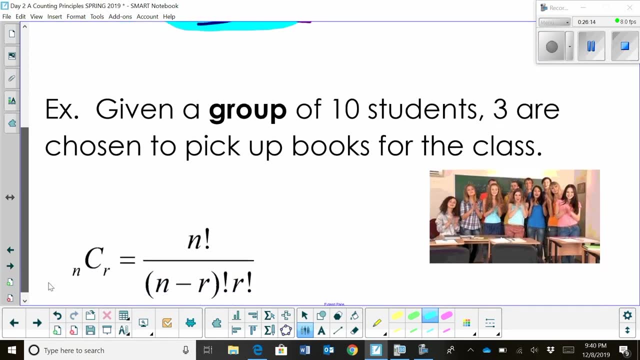 When you're doing a combination, order is not important. You treat it similarly, but you have to read carefully and decide if the order is important. So let's start with this first scenario. Given a group of 10 students, 3 of them are chosen to pick up books for the class. 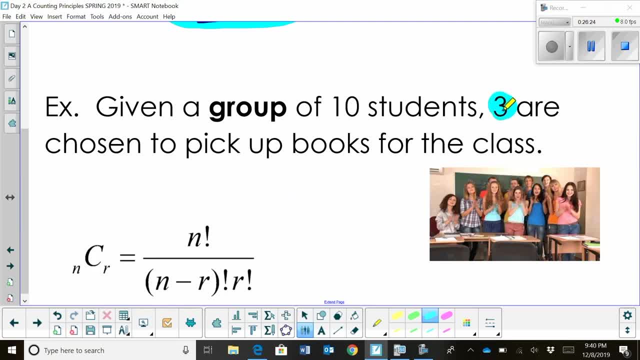 OK, So we're choosing a group of 3 students to go pick up books. OK, That group of 3 is the same group of 3. whether I pick Sally first and Eddie and John, or if I pick John first and then Sally and Eddie, it doesn't matter. 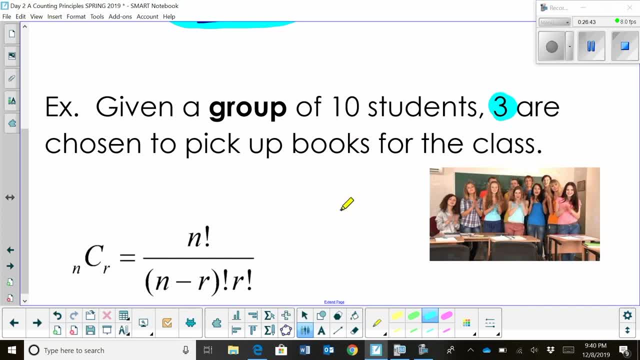 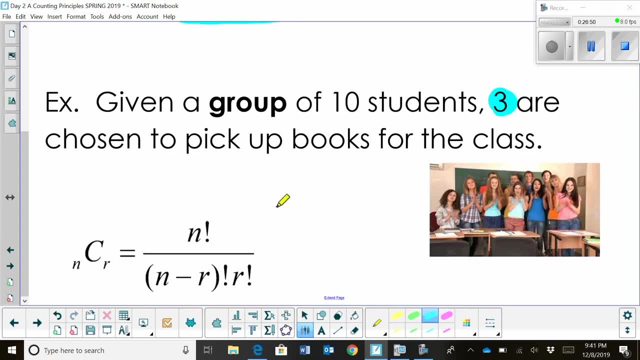 It's one group of students. So anytime you have a group where the order doesn't matter, that one's a combination. OK, so how do we figure it out? Well, we're going to use this little formula for combination. We're going to take n, choose r or ncr, where n is the total number of participants. 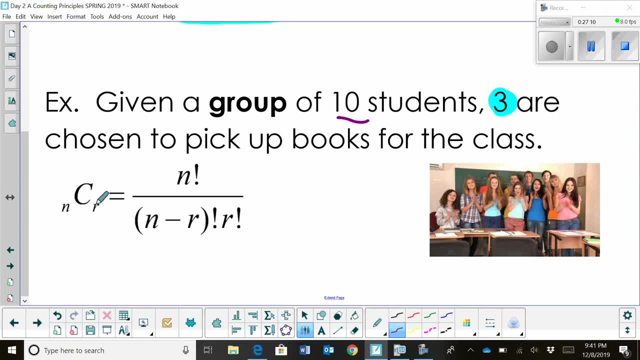 In this case it's 10 students, And then r is how many we're choosing, which in this case is 3.. So this is going to be 10, with a combination choosing 3.. So in our formula we're going to put 10 factorial. 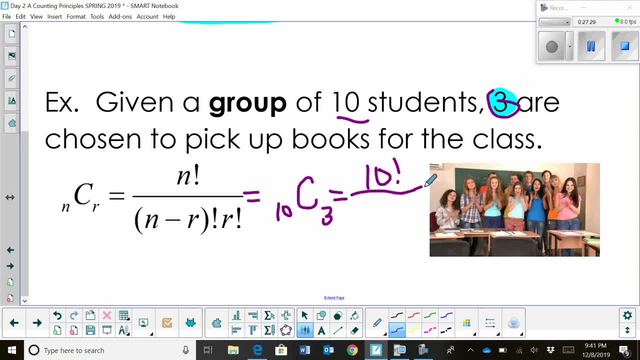 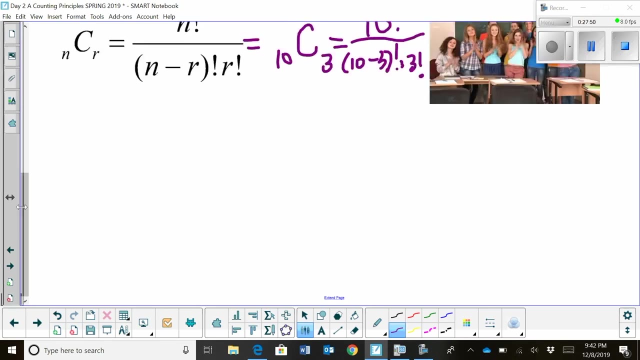 So on top and then on the bottom we're going to take 10 minus 3 factorial, all times another 3 factorial. So we're dividing twice on a combination because we're going to have less possible outcomes than a permutation. A combination is always going to have less than a permutation with the same group and 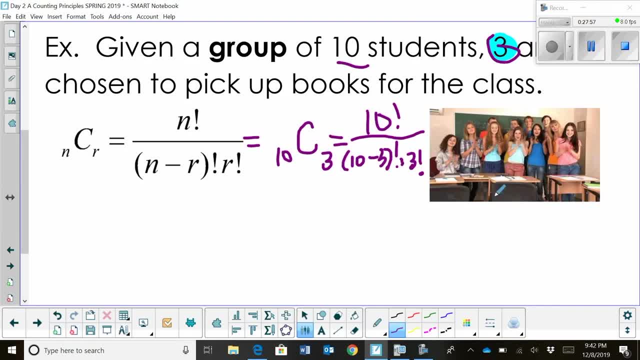 the same choices, Because you're dividing twice and the groups don't. the order doesn't matter And that's why. So take a minute and kind of think through that. So let's write this out. So I have a 10 factorial over. this ends up being a 7 factorial, because 10 minus 3 is. 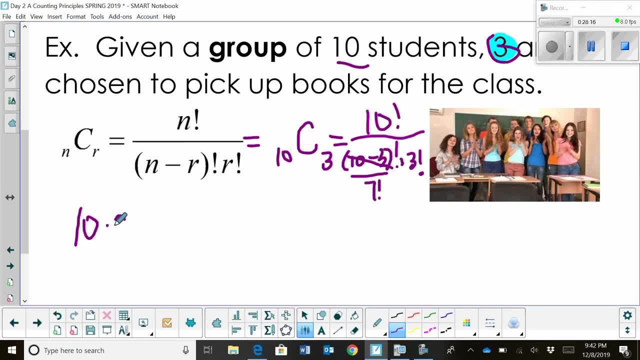 7.. So let's write it out as 10 times 9 times 8 times 7 factorial on top, all divided by 7 factorial, 7 factorial times, and I'm going to write the 3 out, the 3 times 2 times 1,, so we can. 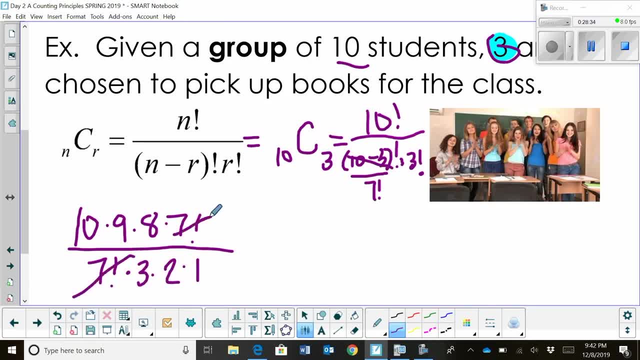 do some reducing. Okay, the 7 factorials cancel, And then I can reduce 3 and 9 just to 3.. And 2 and 8, I can reduce that to 4.. So really, I'm just taking 12 times 10, so that's 120.. 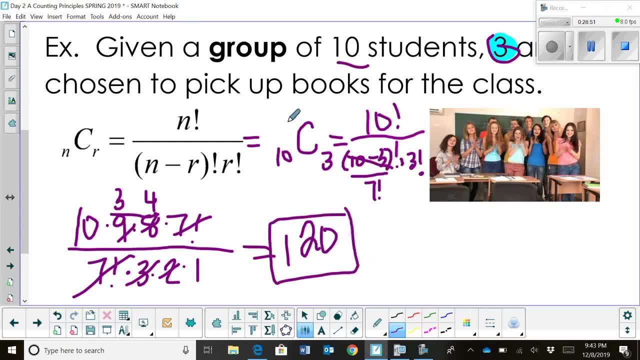 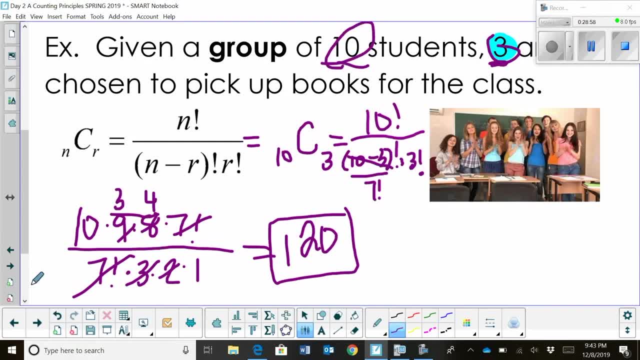 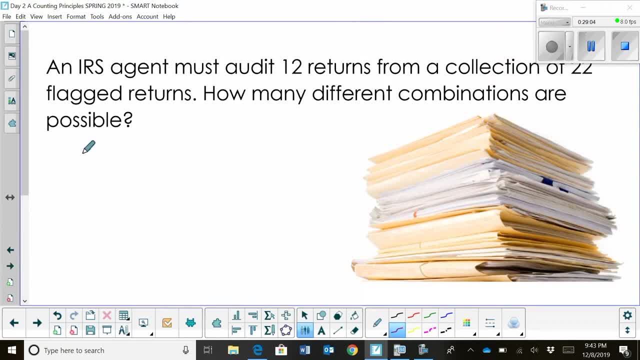 So let's look at another combination. An IRS agent must audit 12 of their tax returns from a collection of 22 flagged returns. How many different combinations are possible? So let's say he's going to get all 12 done today. What doesn't matter if he starts at the top of the pile or the bottom pile to pick the. 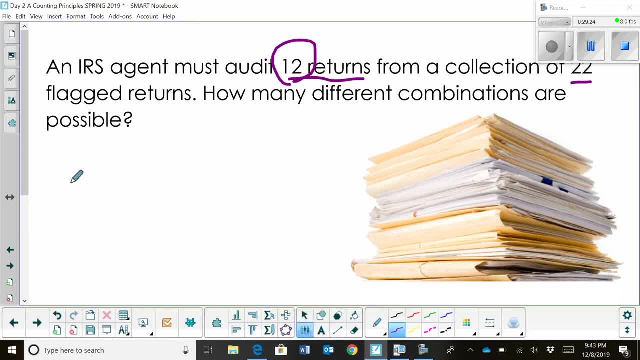 12, he's just got to pick 12.. So what's that going to look like like? well, I've got 22 files to choose from the total number and I'm choosing from there as a combination: 12. so I'm gonna have 22 factorial over 22 minus 12. 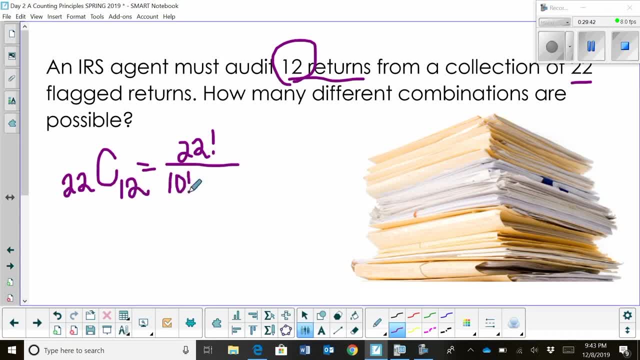 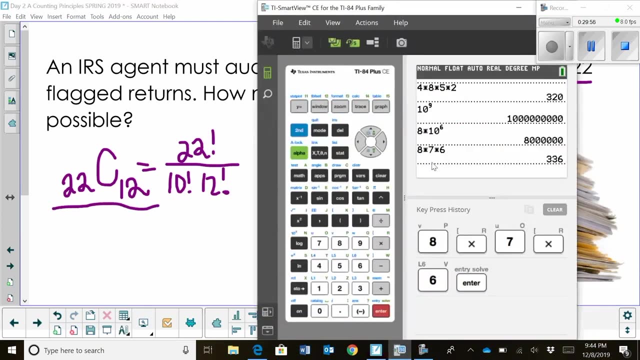 so my difference is 10 factorial times 12 factorial. well you know what? that's a little bigger than I want to handle. so I'm gonna grab my calculator and this time I'm gonna use my buttons- whoops buttons- to calculate that. so I'm gonna. 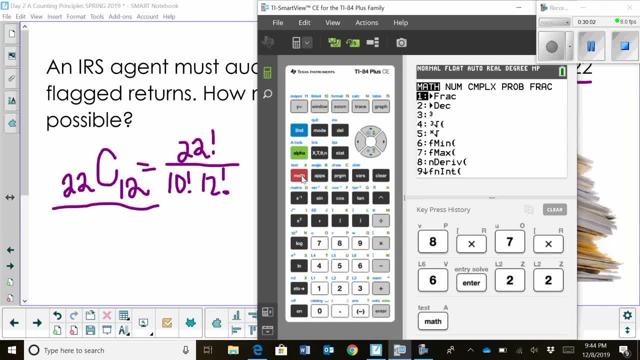 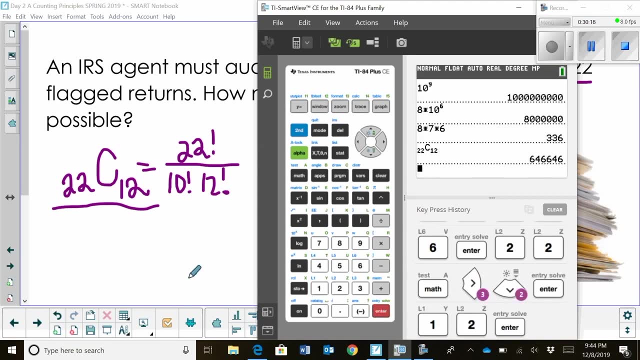 type in 22 and I'm gonna go to the math button, I'm gonna go over to probability, I'm gonna choose, in this case, a combination, and I'm choosing 12, and that means there are six hundred and forty six thousand six hundred and forty six. 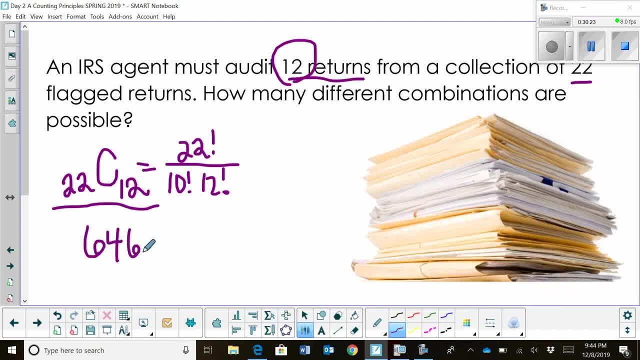 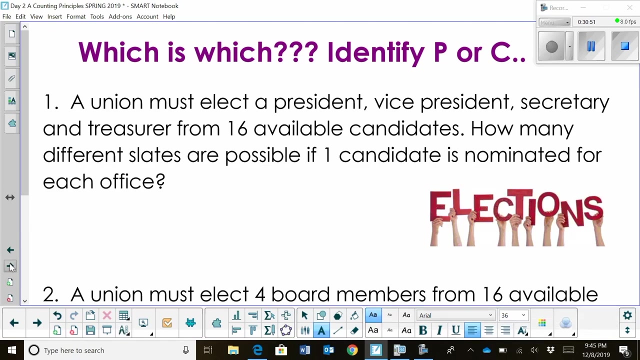 different ways can choose to check tax returns today. that's, and what unit would you put? I would just put ways to choose files. there you go and that's how you figured out. now it's a little tricky. what we're gonna do now in permutations and combinations is try to figure out which is which. which one is a permutation and 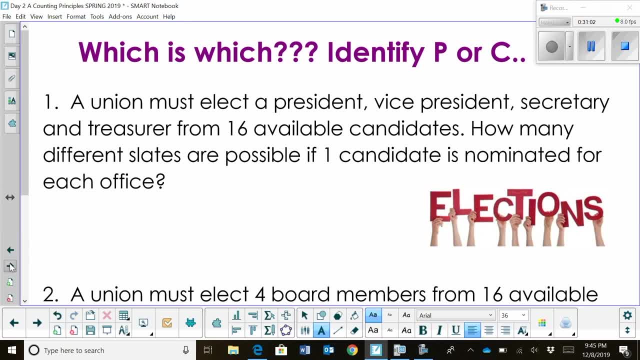 which one is a combination. so we have to read each problem very carefully. so let's look at number one. remember permutation, order matters, combinations, order doesn't matter. so number one: a union must select a president, a vice-president, a secretary, a vice-president, a secretary, a secretary. 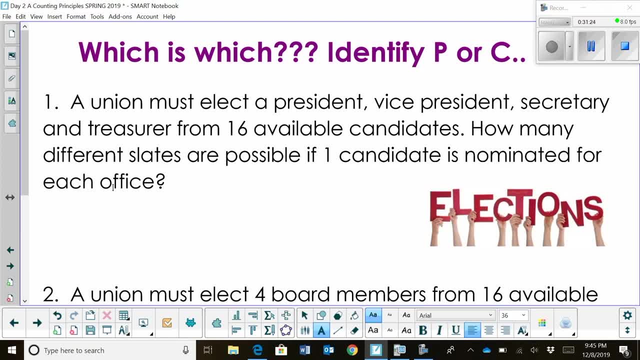 and a treasurer from 16 available candidates. How many different slates of officers are possible if one candidate is nominated for each office? Okay, so you have to think: does the order matter? Does the position matter? And in this case, could I choose four students to be president vice? 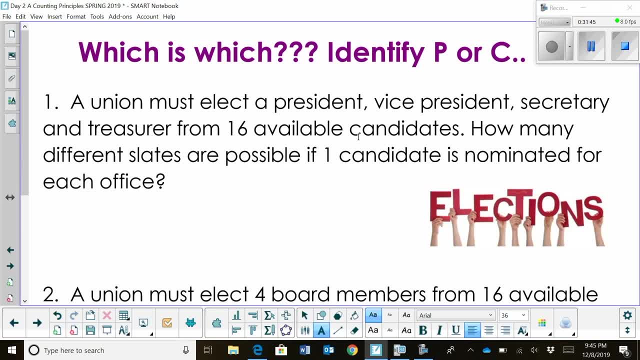 president, secretary and treasurer, and take the four students, reorder them and come up with a new possible slate. And the answer is yes. So this one has to be a permutation. So how would I put it in my calculator? I would do 16 with a permutation of four positions. So let's grab our calculator. 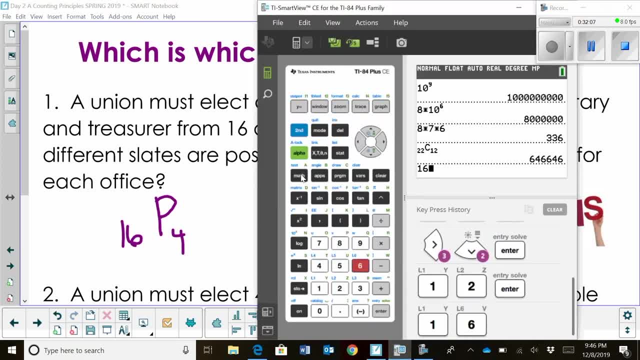 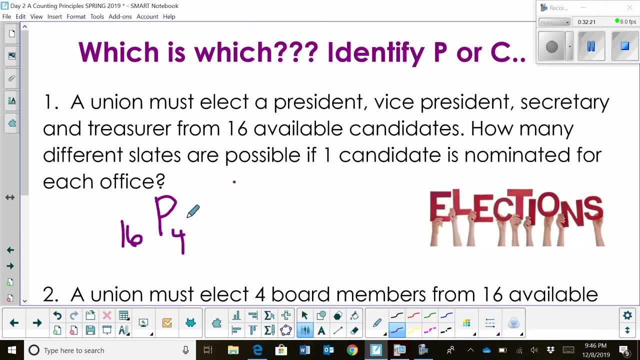 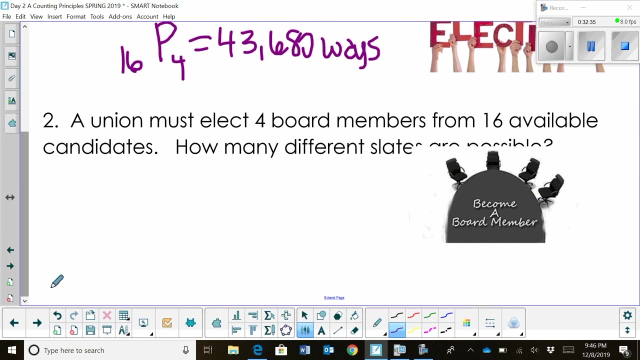 and do 16, math probability permutation this time. and I'm choosing four positions And that's four. So this one has 43,680.. So this one has 43,680 different ways to choose for the election. Okay, so let's try the next one. A union must select four board members from 16 available. 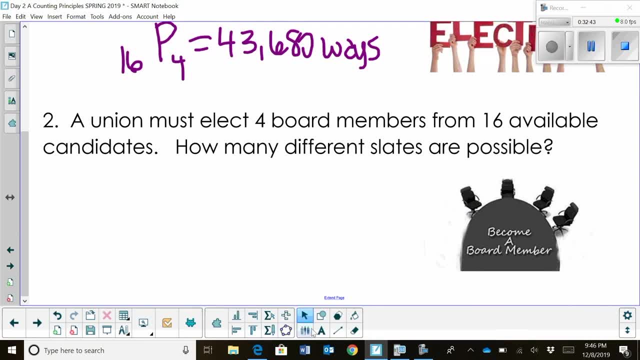 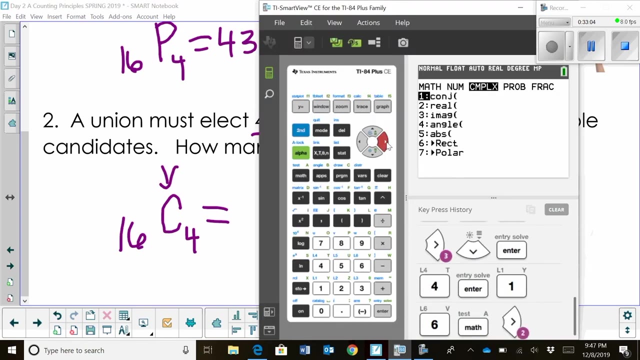 candidates: How many different slates are possible? Now, this one's different because we just have board members. They're not assigned to a position, So that one is a combination. So I'm going to do 16, choose four. but this time it's a combination, So let's do 16, math probability: choose a. 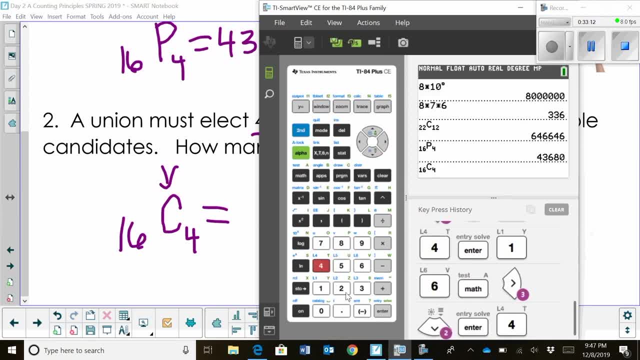 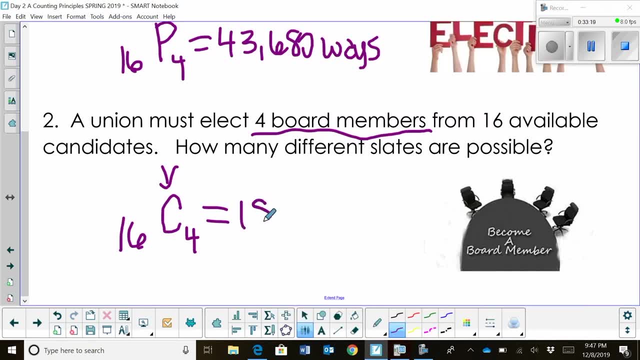 combination and choose four. Now the combination will have less possibilities. It's only got 1,000 and 820.. And why is that? Because the order didn't matter. The same group of four aren't going to be assigned to a position, So that's how we can do it. Okay, so let's look at a summary kind of of. 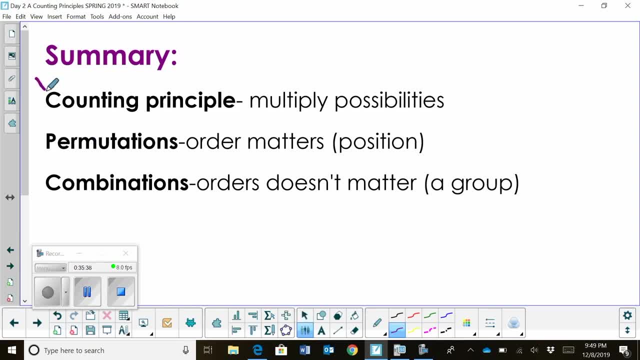 what we did. Okay, first we looked at the counting principle, And that's just when you look at different ways to choose from, like a menu or maybe an outfit from a group of clothes, different ways you can do it. So let's do 16, math, probability, choose four And that's the.